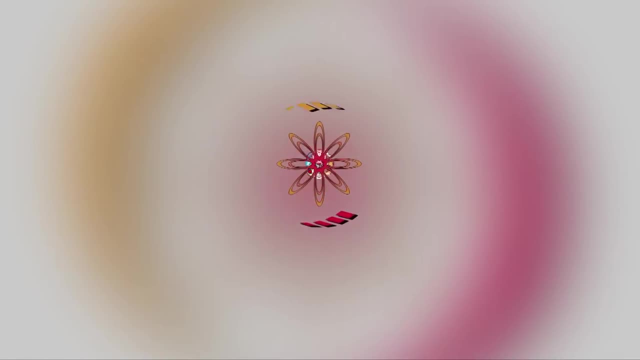 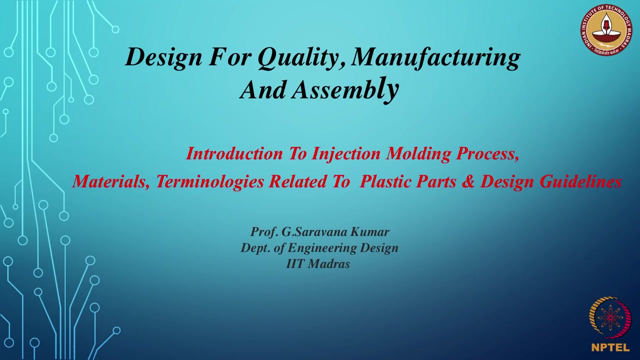 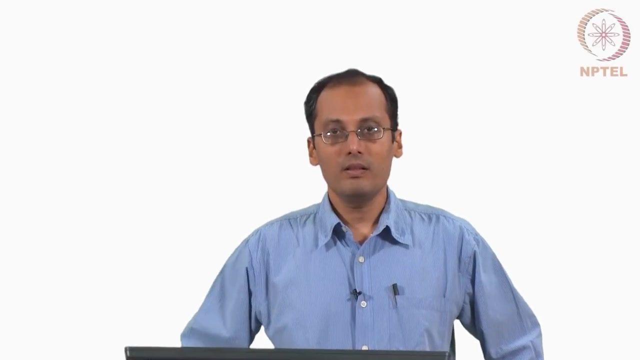 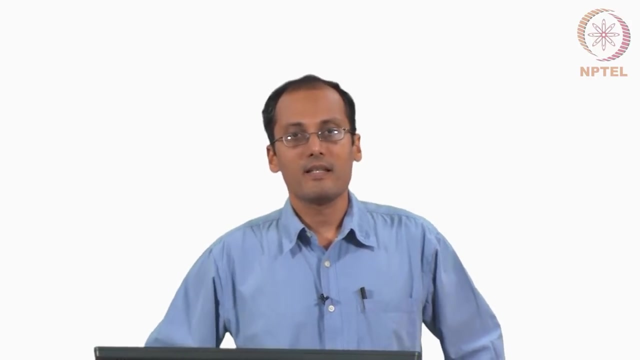 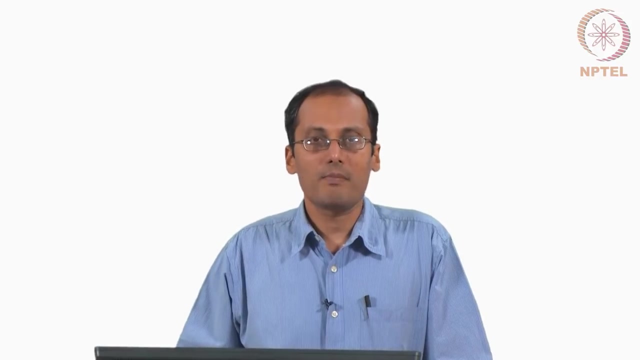 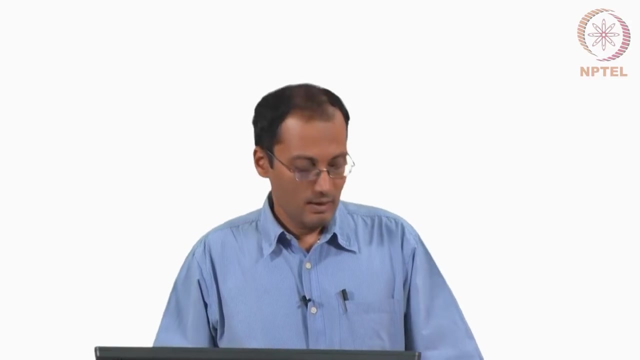 Good afternoon everyone. This course is on Design for X and as part of this course, I am going to discuss design for manufacturability, specifically that of plastic parts, in this lecture. So I am Saravana Kumar from Department of Engineering Design, IIT Madras. 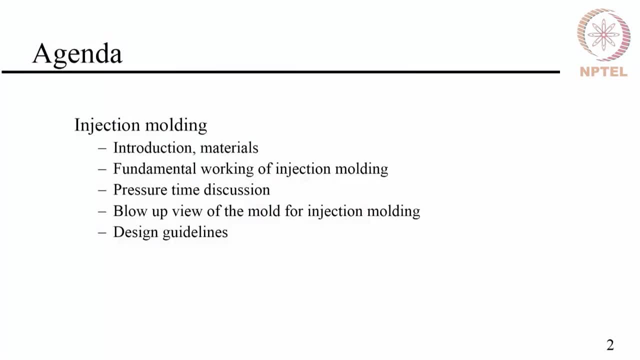 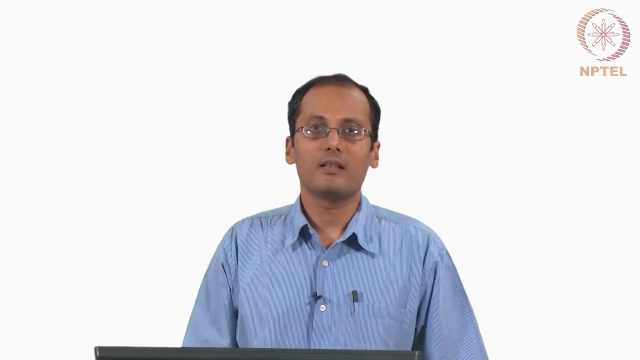 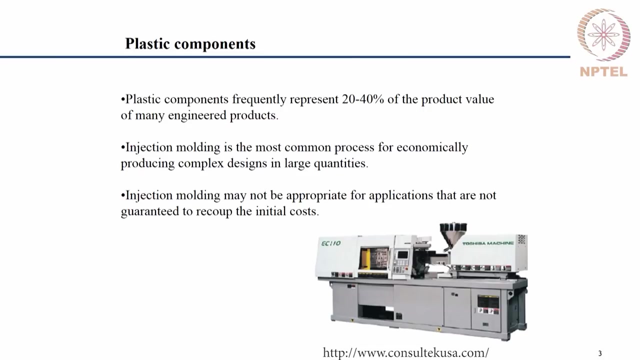 So this is agenda for today's lecture. So we will see the injection molding process which is used predominantly for manufacturing plastic components. We will see the process, the materials and the design considerations for plastic parts. So plastic components are majorly used in most domains, about 50 percentage to 60 percentage. 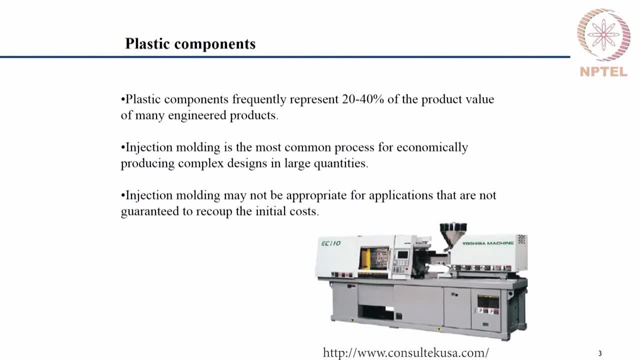 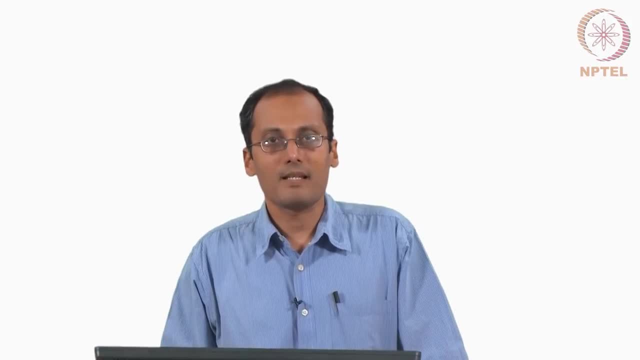 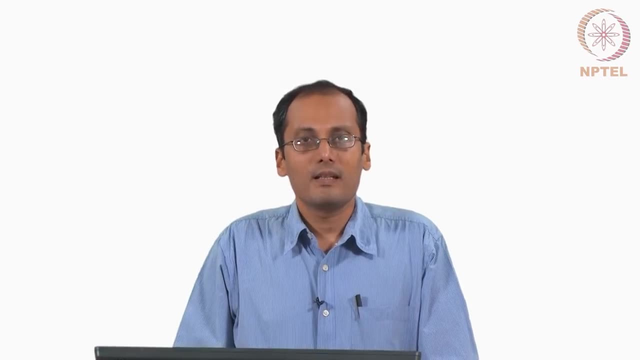 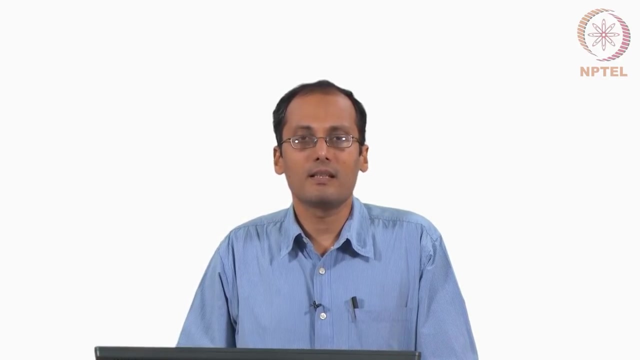 of the components used in various sectors, whether it be automotive or biomimicry, These biomedical or household appliances. they are made from plastics. As plastic materials are used extensively, the manufacturability and the cost of the product is significantly affected by the manufacturability and the process processing of the plastics. 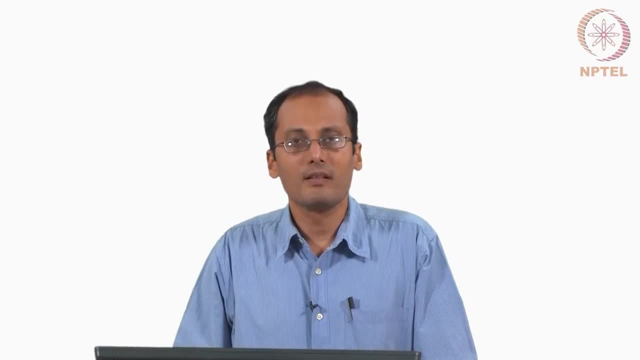 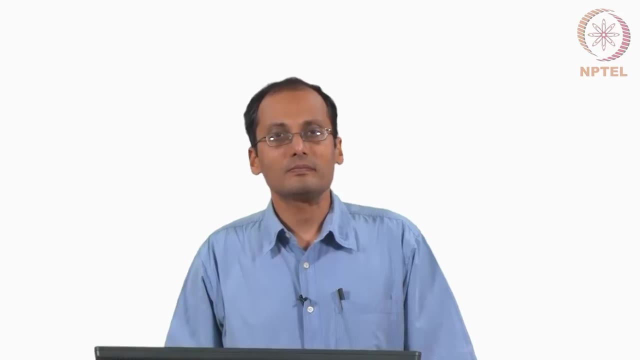 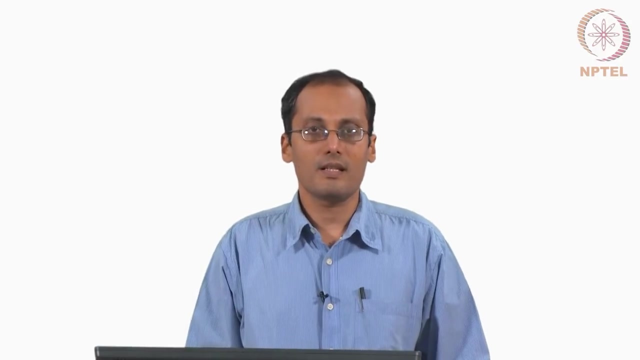 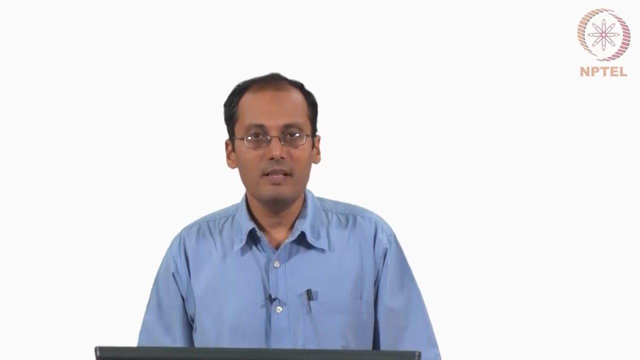 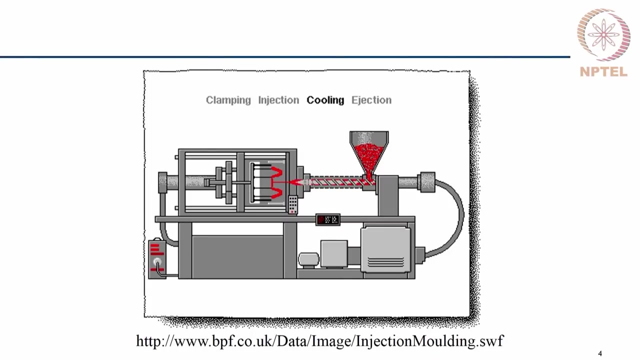 So injection molding is one of the processes that is predominantly used for making the plastic components, because for large volume production the cost per piece is the least for the injection molded components. So injection molding process consists of about 4 stages: The mold, which confines the material to the part geometry. 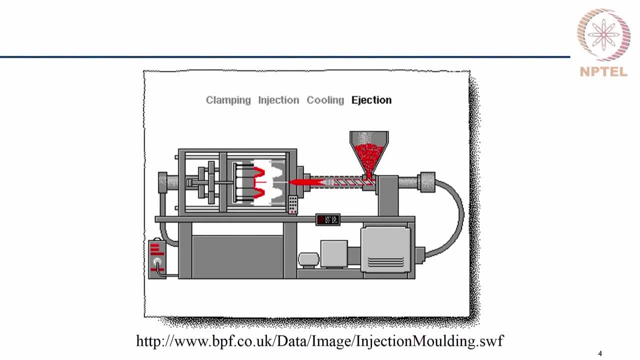 It is made from the part drawing and mold is manufactured and the mold is clamped using the machine. So there is a movable part of the mold and there is a fixed part on the side from which the injection takes place. So you can see that. 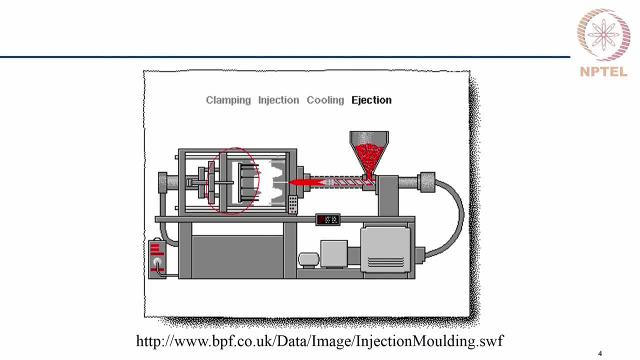 This is the moving component and this is the fixed part of the mold. and once the mold is clamped, the injection takes place. The plastic material is injected by the injector. Once the material is filled in the mold, it is allowed to cool and finally, the part is. 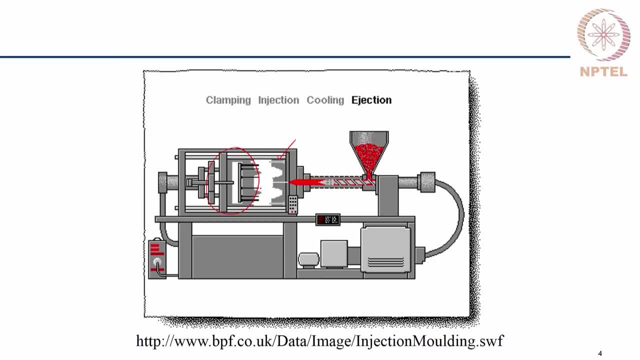 ejected. So this constitutes one cycle of molding, And the time that is required to complete one cycle determines the cost of the part. So the optimization for the process involves reducing the cycle time. One of the important parameters is the cycle time. 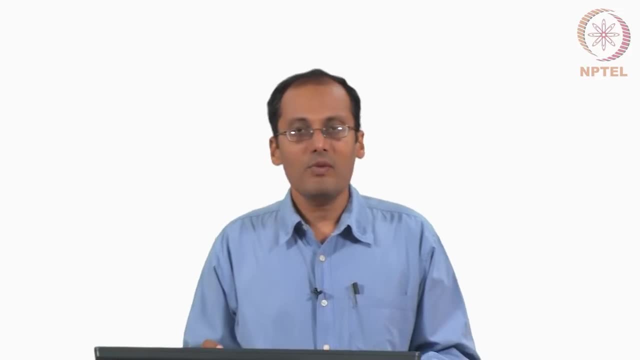 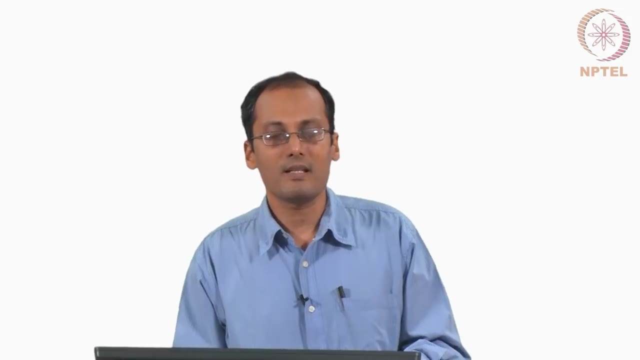 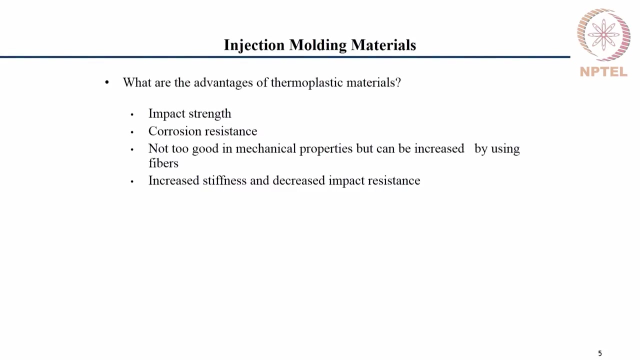 So as thermoplastic materials, they are quite versatile And there are a lot of engineering grade thermoplastic materials that are used. They can be used wherever there is chemical and corrosion resistance is required. where we need good strength, we can use it. 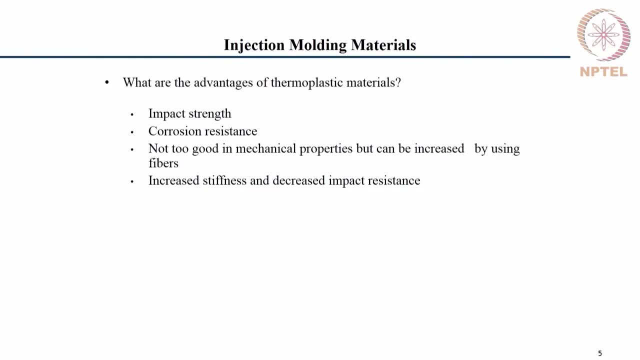 And the limitations in terms of the usage comes from the fact that they cannot be used for very high mechanical loads, So they cannot be used for very high mechanical loads. So they cannot be used for very high mechanical loads And also for very high temperature applications. 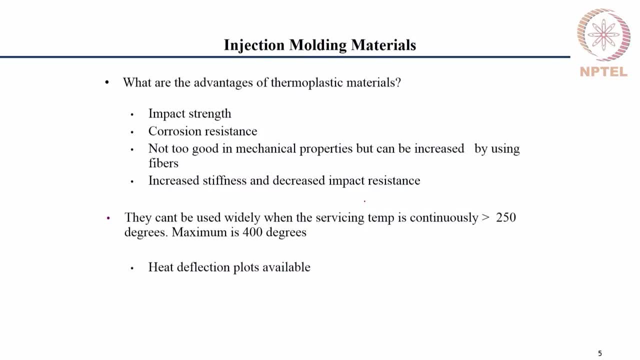 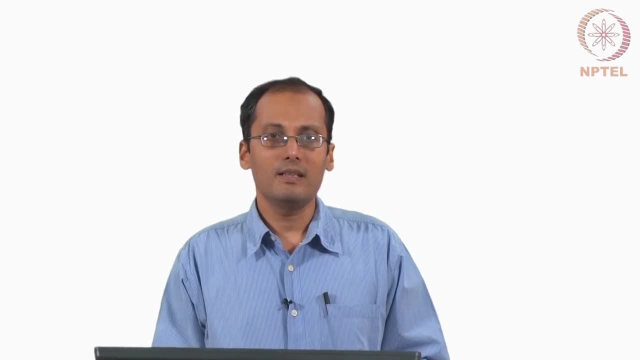 Typical usage temperatures are up to about 200 degree Celsius and there are some grades of plastics which can serve at slightly higher temperatures. So the heat deflection plots for different materials are available as design materials. So the heat deflection plots for different material are available as design guidelines. 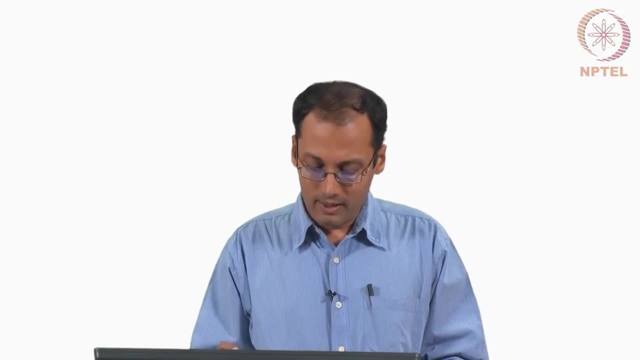 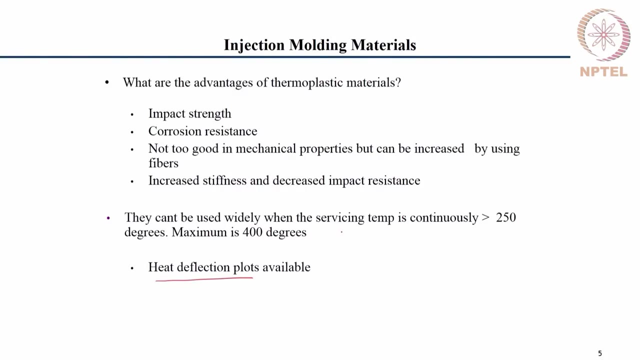 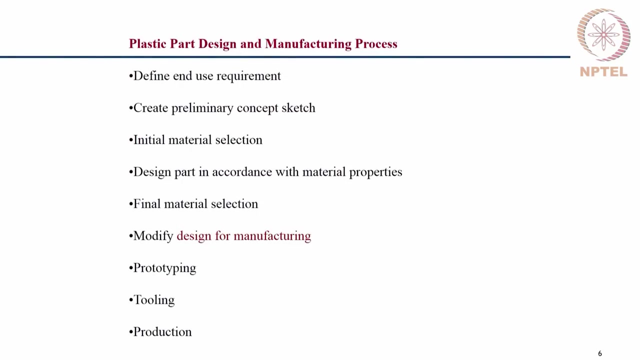 which are used for making the choice of the material If there is a requirement for service temperatures at a higher degrees. So a plastic part design and manufacturing process starts with defining the end use requirement, because that decides the type of material that needs to be used. 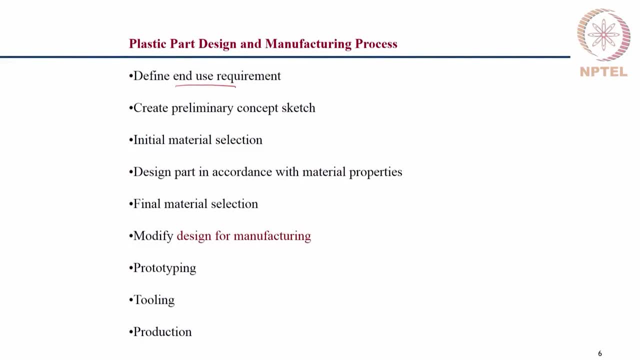 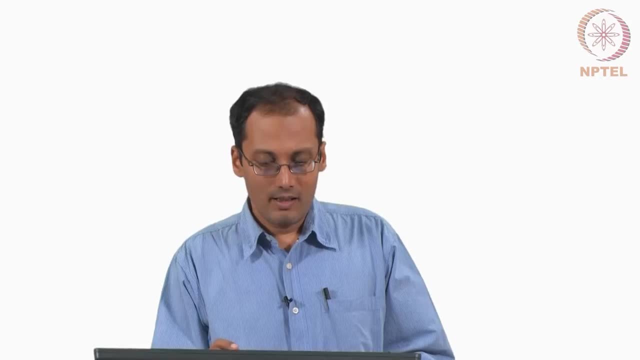 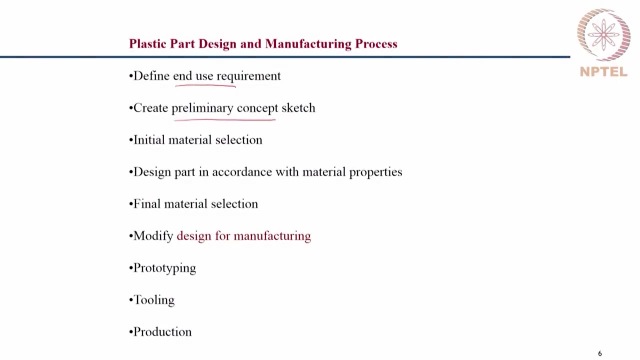 So the plastic part design and manufacturing process. we have to start with defining the end use requirement, because that decides the type of material that needs to be used for theseason to be used and the process for manufacturing the same. Based on the functional requirement, a preliminary concept is generated, a design concept is. 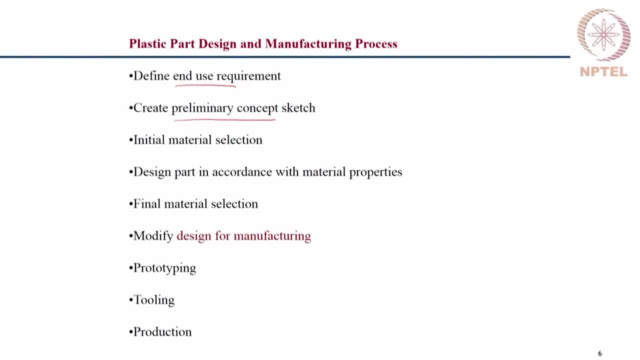 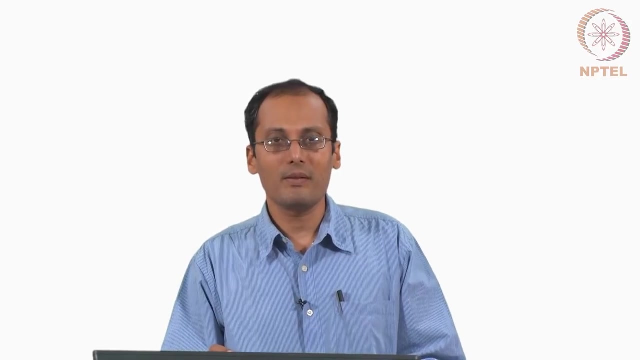 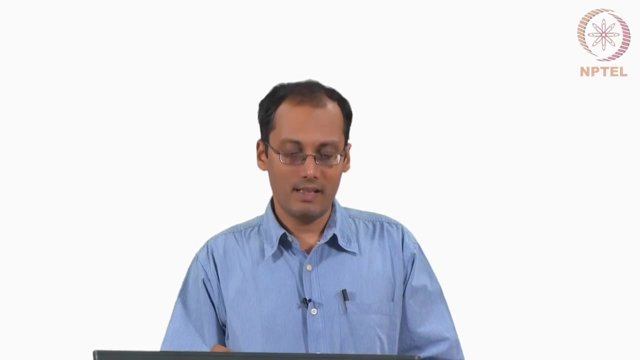 generated and material is selected and the part design is made according to that. So this is an iterative process, because once a material is selected and a design is made, various functional testing, either in computer simulations or by using prototype, and verification is done before the material, as well as the design, can be finalized. 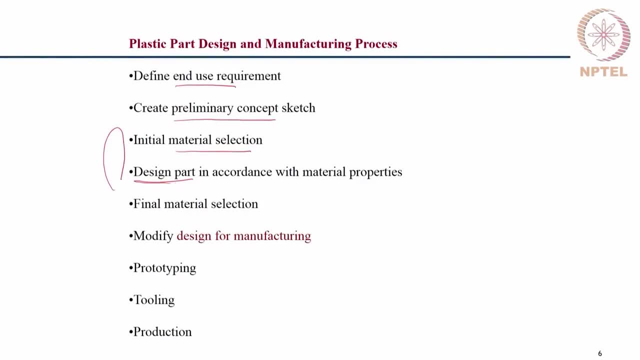 So this step itself is highly iterative in nature, And also we consider manufacturability and the cost, and this step is also iterative. So we will see what are the design considerations for manufacturability, for the injection molded components, And once the design is fairly matured we go ahead with prototyping and then developing. 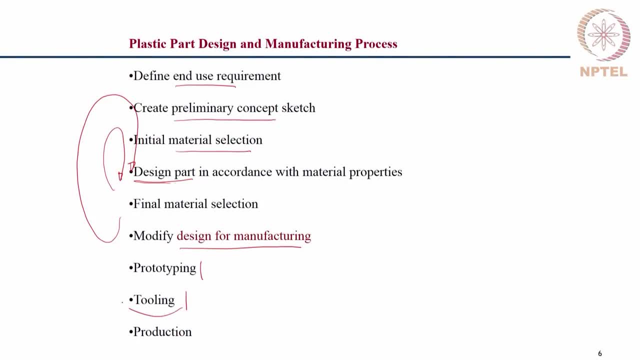 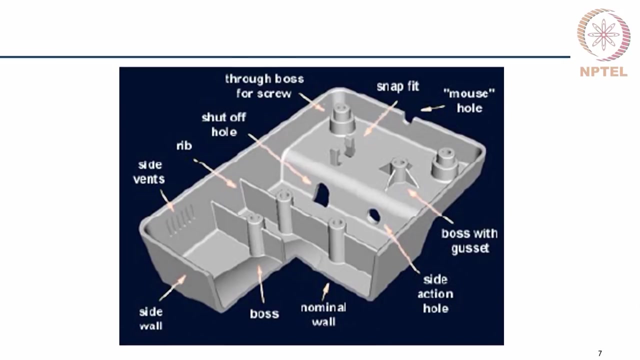 the final tooling, Because here So we are making the tool and thereby we are incurring the cost. So this step is very critical. we cannot typically go back to design when we are here and then we release the mold for production. 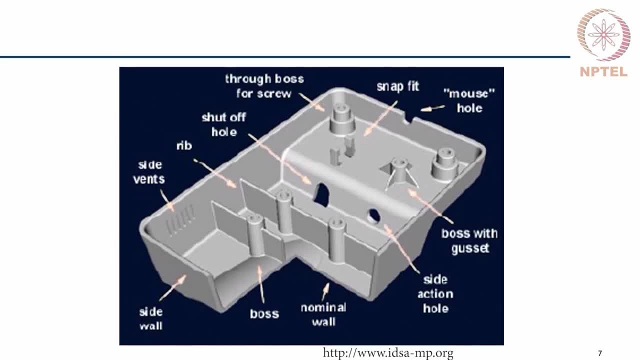 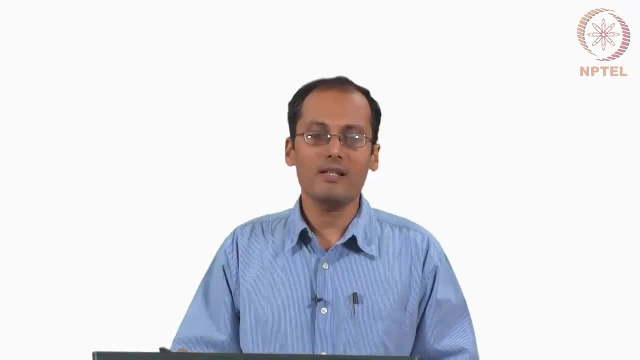 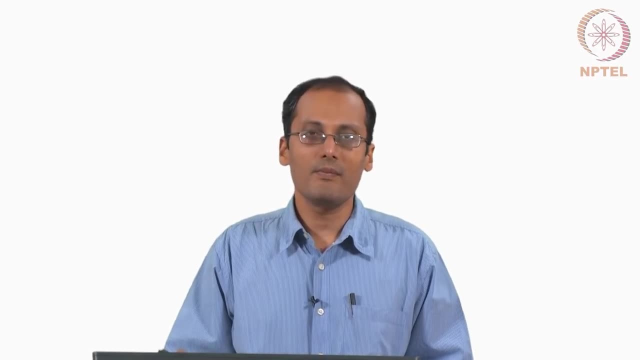 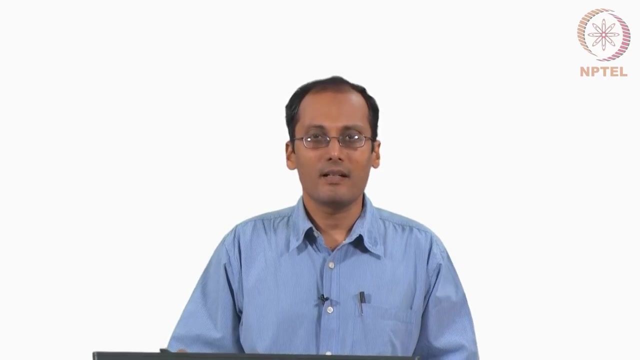 Before we see the process, let us understand certain terminologies associated with plastic components. Typically, plastic components are made of the same material. Typically, plastic components are thin components, shell like structures, and for stiffening the structure we use ribs and webs and bosses wherever we need to have some interfacing. 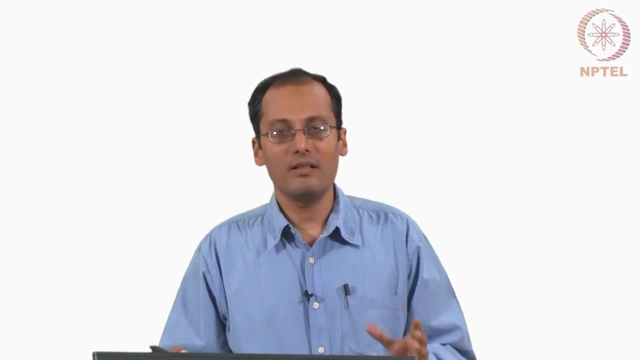 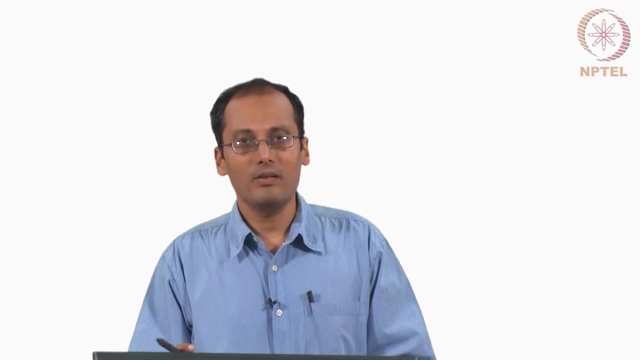 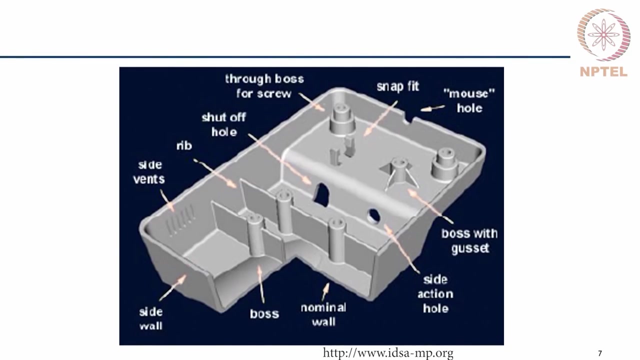 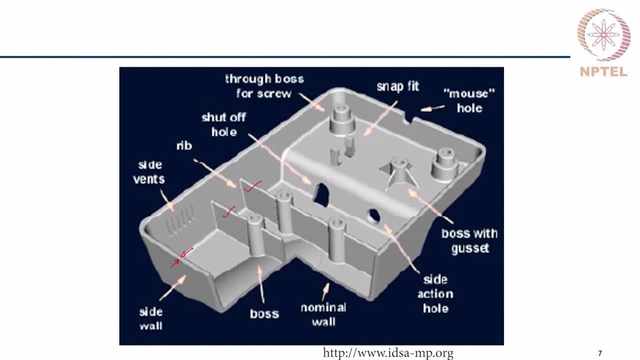 adding too much weight And we have the bosses, which can take in elements like screws. The bosses may also have sometimes these gussets to provide additional stiffness And sometimes the bosses may be made thicker or they may be through bosses to accommodate screws. 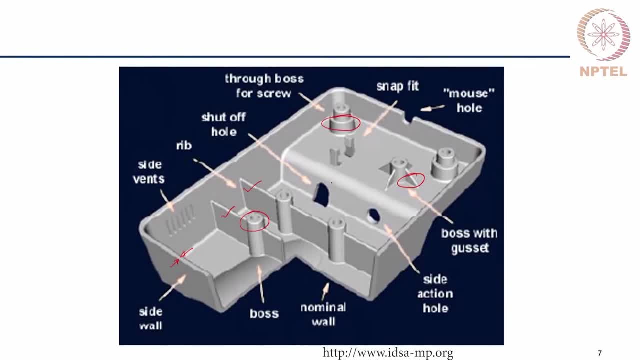 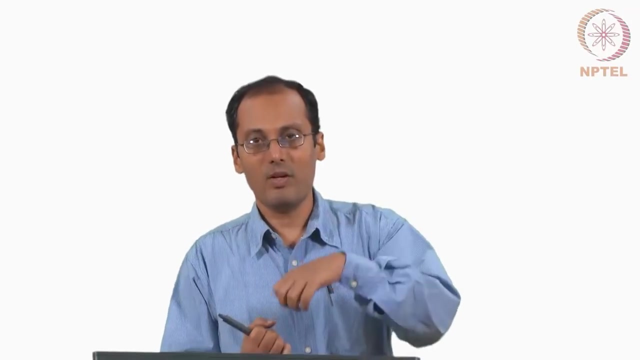 There may be holes like this shut off hole that you see over here, or these mouse holes. So these holes, as you can see, they are on the transverse direction. The injection molding direction for this component is from top to bottom. that is the mold action. 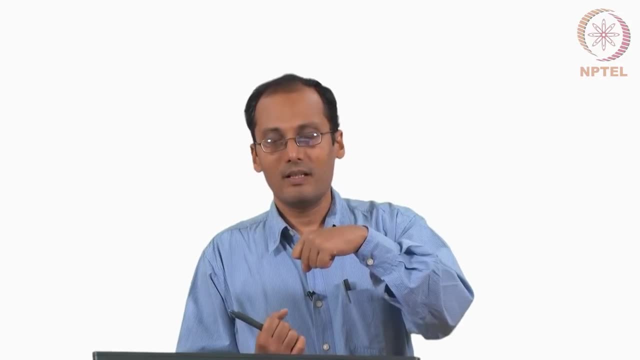 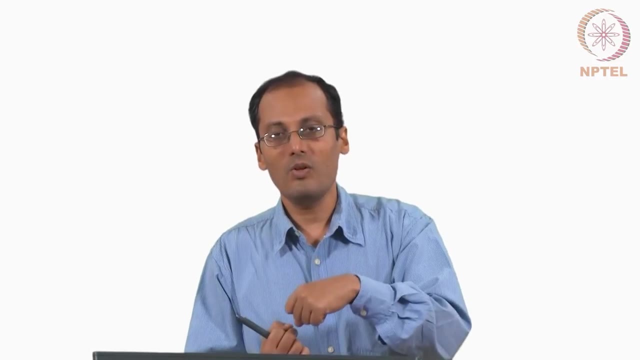 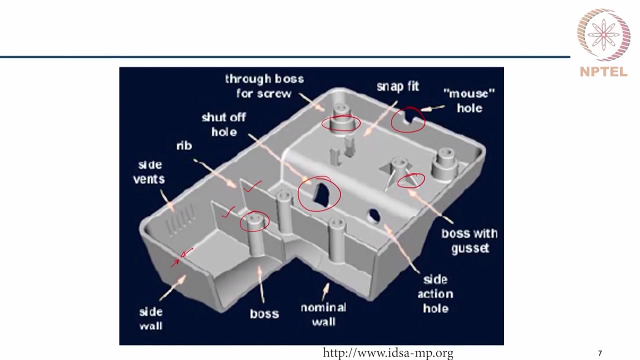 takes place from top to bottom and the part is taken out. So all the features that are along this mold opening and closing direction- So they are these side walls, the ribs that you see in the picture, as well as the bosses, The features like this mouse hole and the shut off hole and the side action hole, they 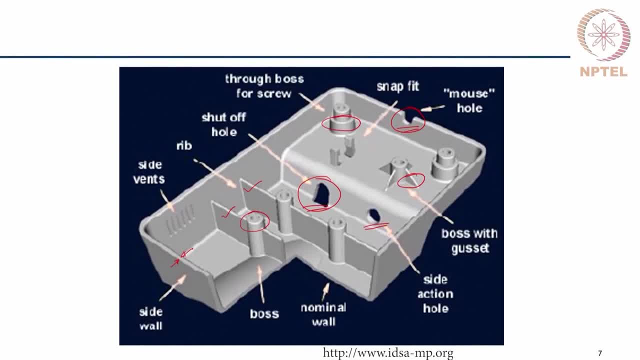 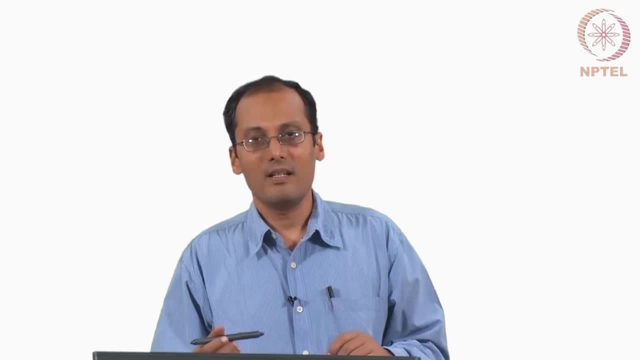 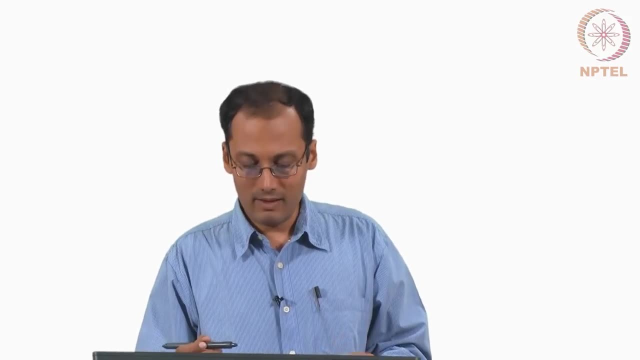 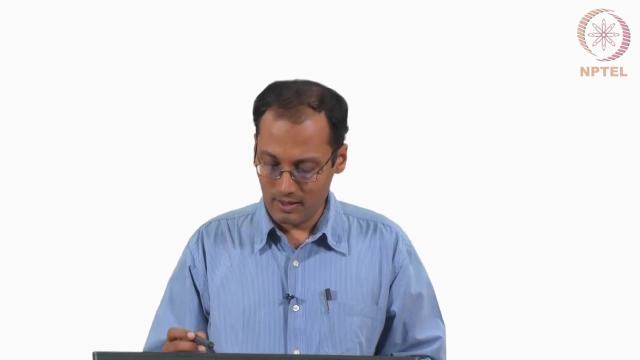 are transverse to the mold. Ok, So there should be some special structures in the mold, like what we call as a side action pin, So that these features can be created in the mold and the part will have these features. Once we see the whole process, we will be able to appreciate the need for these side action. 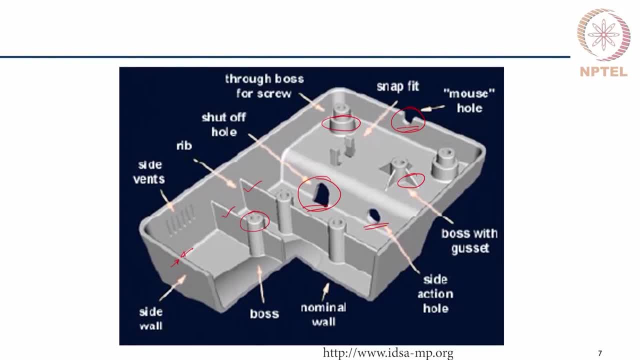 pins. So these holes like the shut off holes, So these holes like the shut off holes, So these holes like the side action pins, So these holes like the side action pins, So these holes like the shut off hole, can be made using a mold feature in the mold opening. 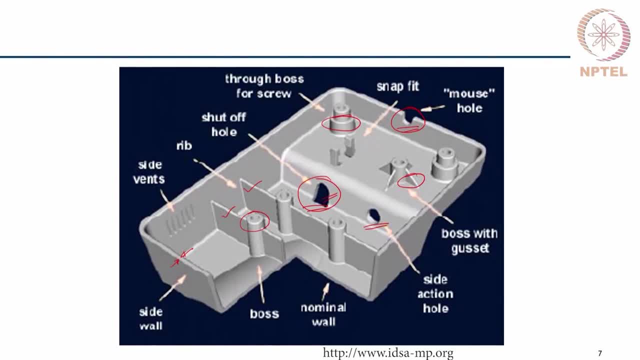 and closing direction. but this side action hole needs a side action pin. Even this mouse hole can be made without side action, because that can be placed just along the parting line. This is the parting line, So this feature can be obtained without side action. 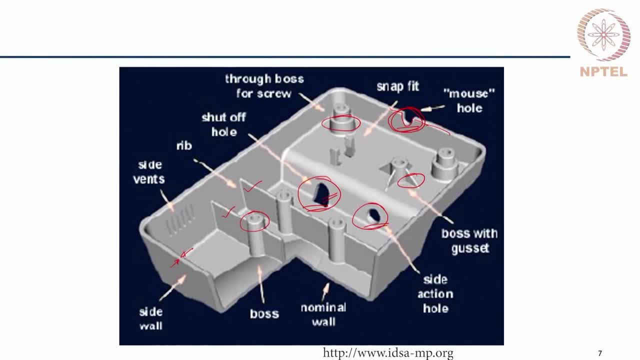 Ok, Without having a side action pin in the mold. So these are some of the terminologies that we may be referring to as we discuss. We also see one feature here. this is called as a snap fit feature. Most of the times in plastic components we try to avoid to the extent possible the screws. 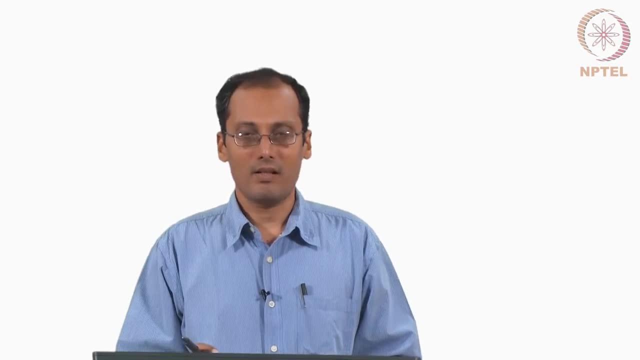 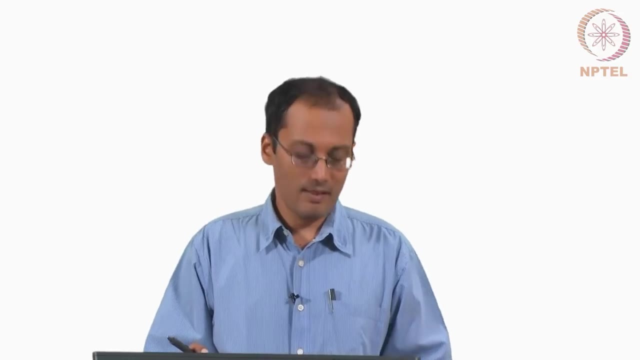 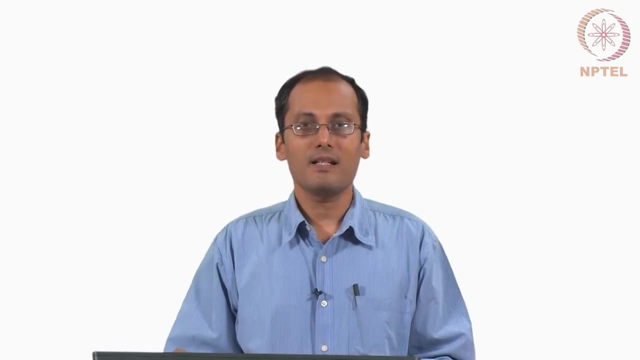 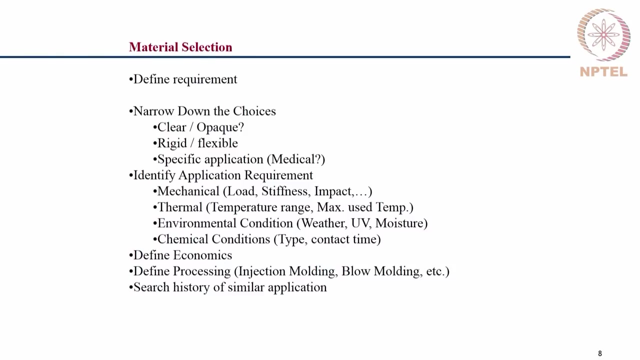 and snap fits are encouraged because that reduces the assembly time When these components are in the mold, Ok, When these components are assembled with other structures. So in this process, the material section selection is the key and the first process. So there are several choices to make based on the functional requirements, such as whether 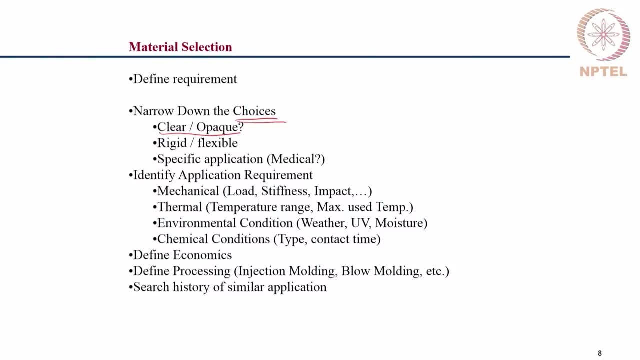 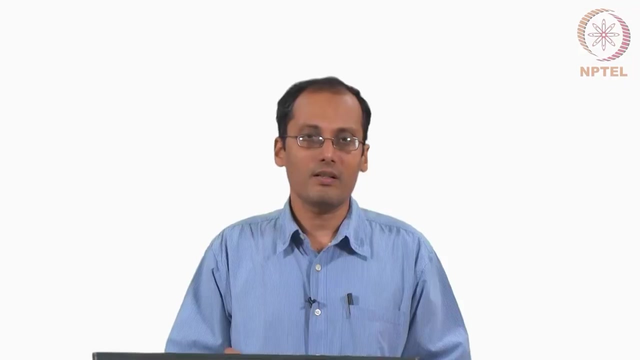 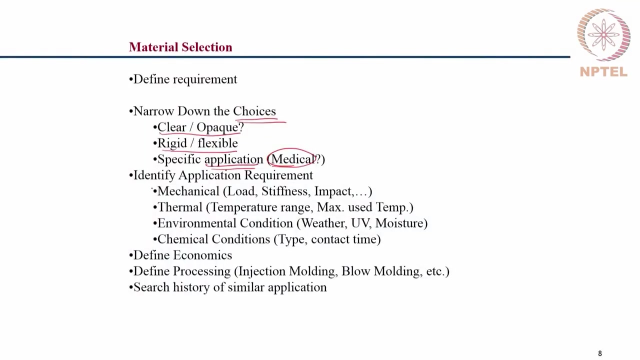 the component that is being made should be clear or opaque, Ok. Or whether it has to be rigid or flexible. What is application Applications like medical needs, special types of plastics? there are FDA approved grades of materials used for medical applications and based on the functional requirement, what? 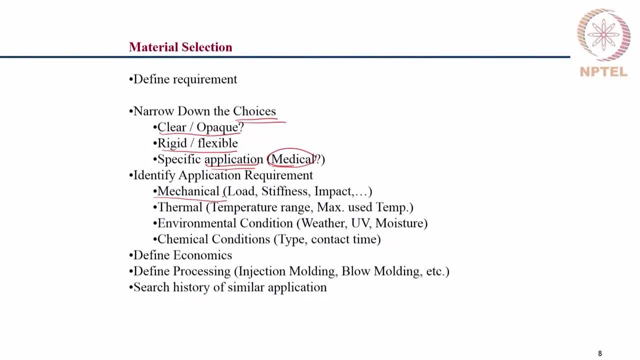 kind of loads? Ok, And impact will come on the component. what kind of thermal loads will be there, like the working temperature, maximum temperature, the environment in which this component will be servicing, like the humidity, weather, UV light and so forth? 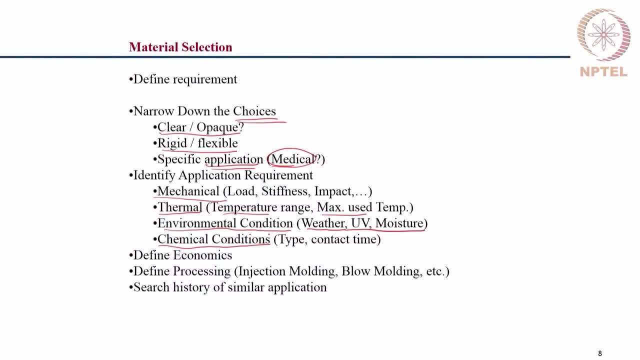 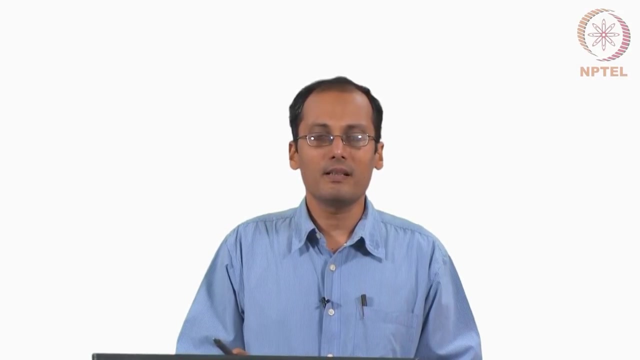 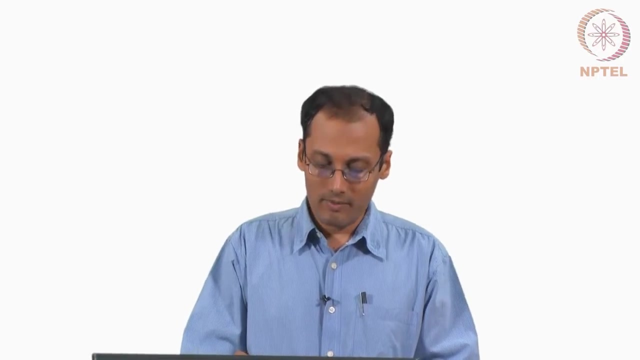 Also the chemical nature of the environment is to be considered. Ok For doing the material selection. Material selection also should consider economics, because one of the key characteristics, are one of the significant parameters associated with the plastic part design is the final cost. So economics is important. 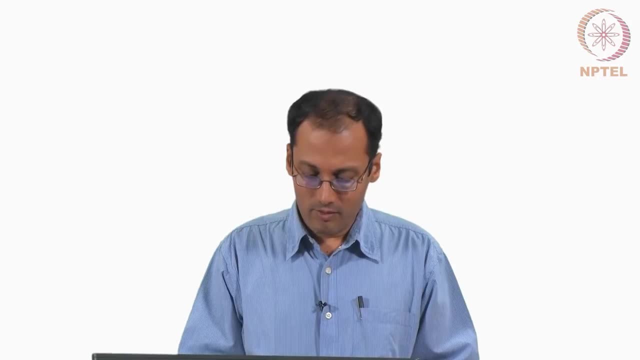 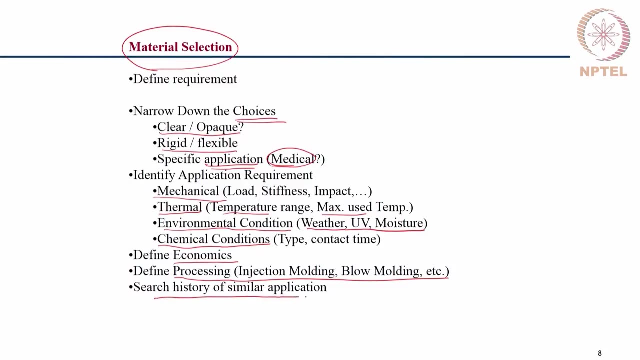 And based on this, Ok, We have to also look at the processing condition and take help from history in terms of applicability of the material for similar applications. So this is a guideline for doing a material selection. So there are lot of materials that are available. 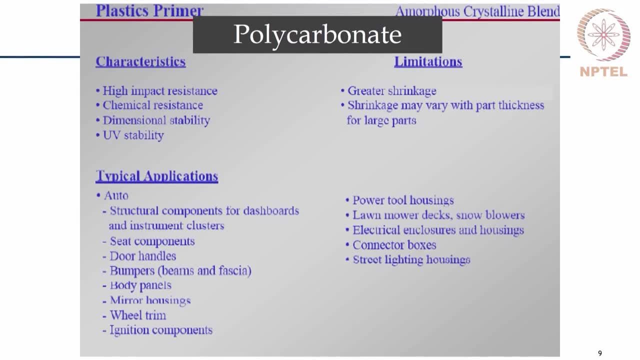 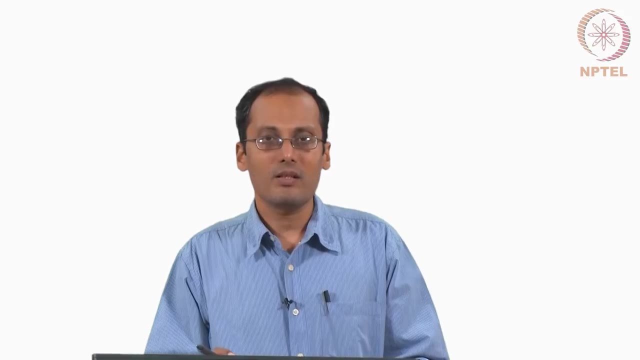 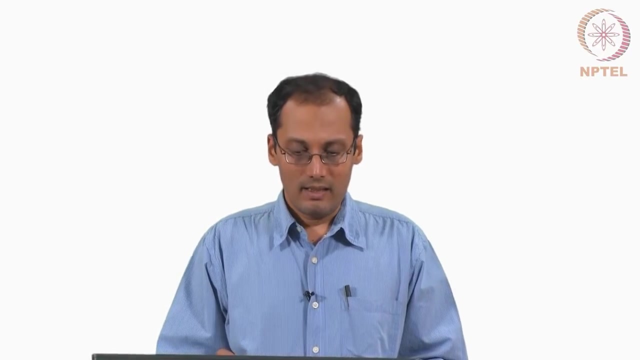 There are guidelines available for choosing the material. Ok, So there are a lot of materials that are available. So there are guidelines available for choosing the materials based on the various characteristics. Few sample materials we will see. So one of the most used materials is polycarbonate, or in short, we call it as PC. 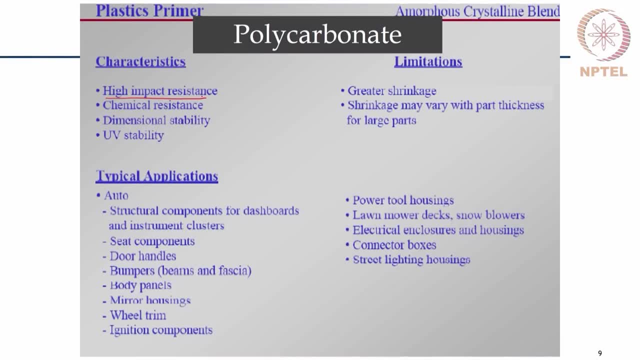 It has very good impact resistance and dimensional stability. apart from various other positive attributes, It is predominantly used in automotive structures wherever strength and impact resistance is important, like door handles, body panels, etcetera. Some limitations in terms of the shrinkage: the part shrinkage needs to be considered. 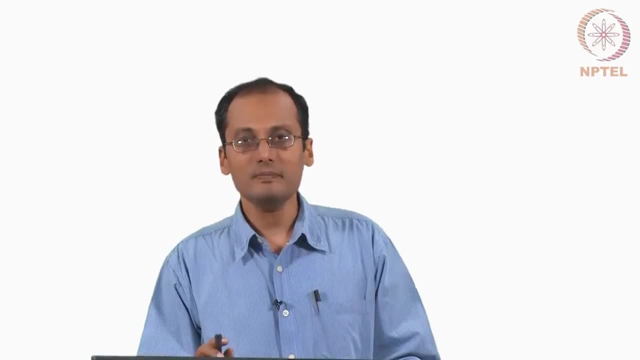 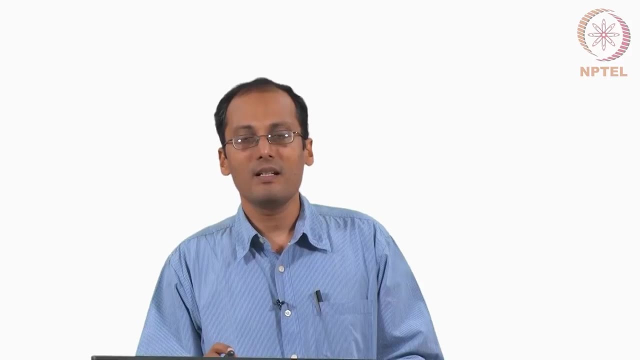 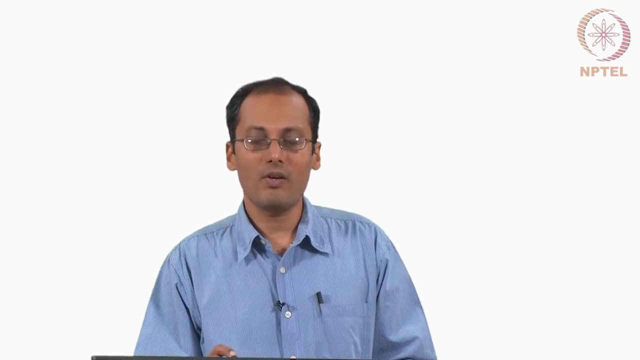 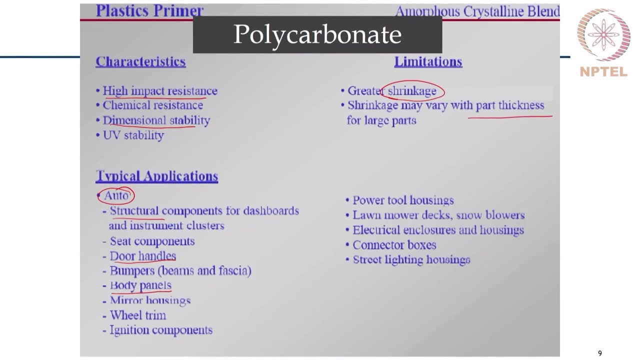 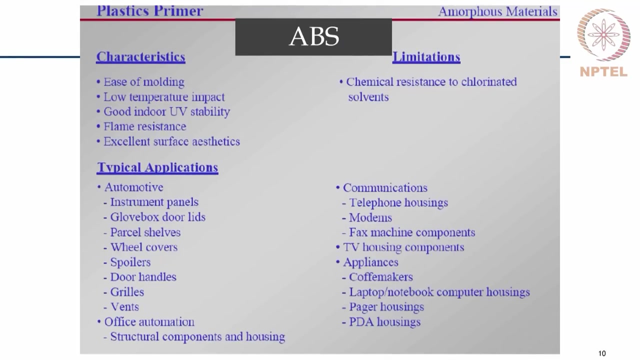 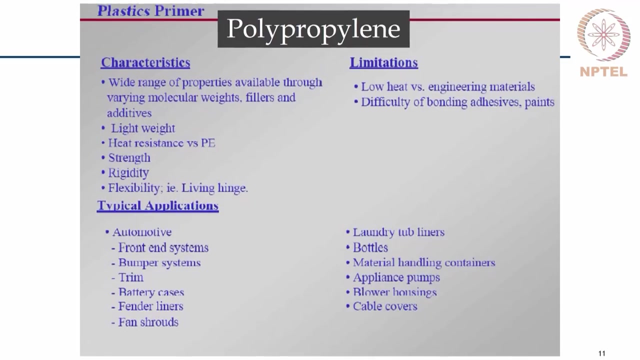 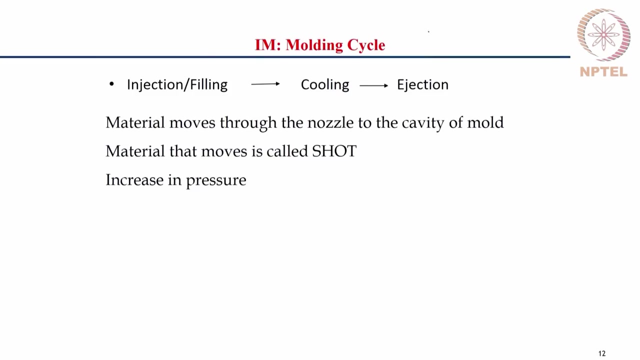 while designing the mold. So the chemical resistance to chlorinated solvents is less. So based on these considerations, one can choose the material. One of the other important material is polypropylene, or what we call as PP. 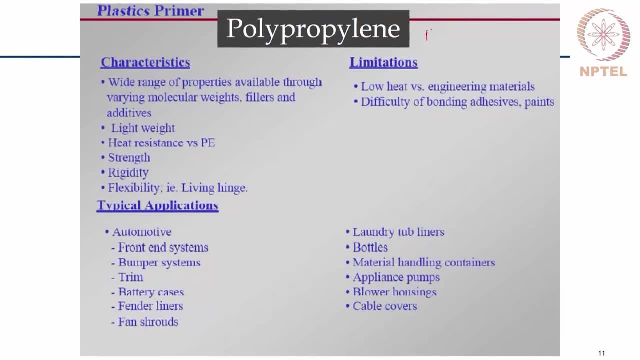 It has lots of applications, particularly because of the requirement wherever there is a light weight requirement and the flexibility A lot of casings and liners shrouds, and all are made using this material. In terms of limitation, it cannot be used in mold. 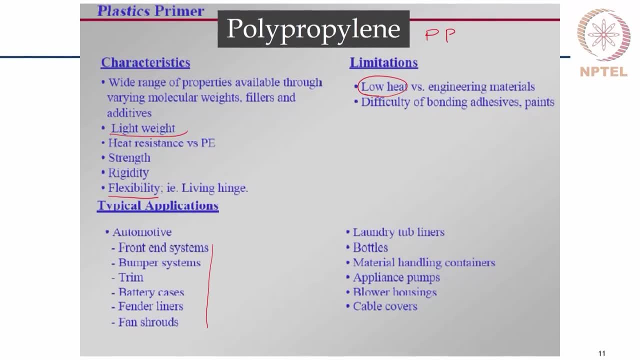 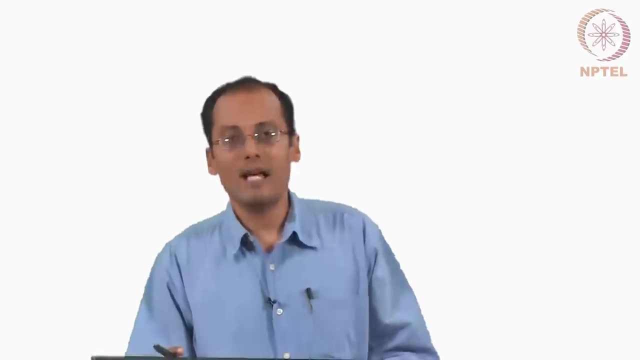 high temperature or wherever there is lot of, you know, use of materials for bonding and difficulty in painting. So lot of other applications like bottles, water bottles to laundry tub liners are made using this material. So this is just a sample of the spectrum of materials. the thermoplastic materials: 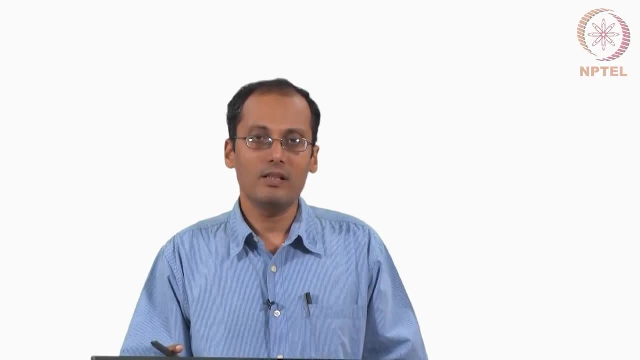 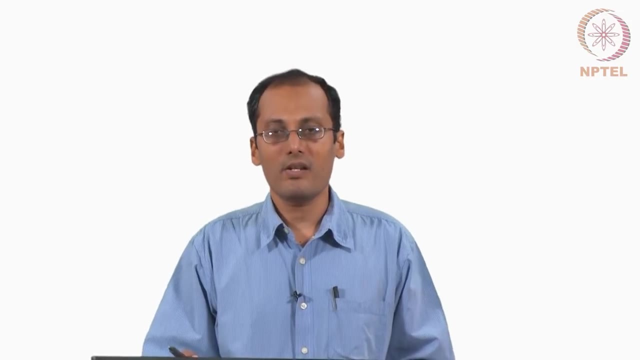 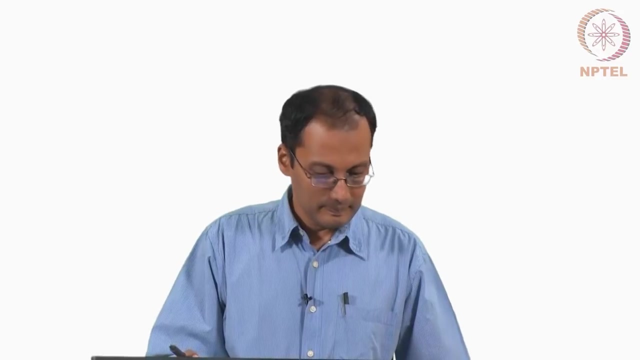 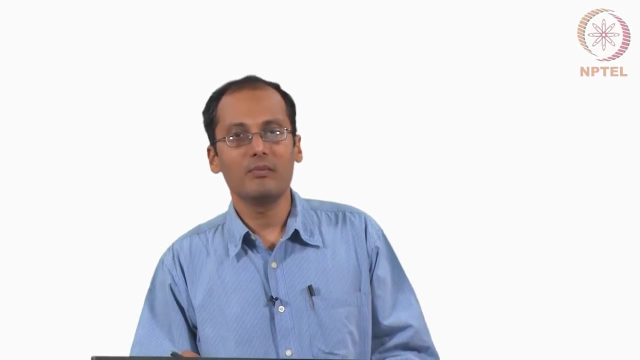 that are available and there are good material selection guides available to help engineers make the good initial choice of material and then iterate upon based on the design and the requirement. So once the Material is selected, we need to make the mold. and in order to design the mold, we need to. 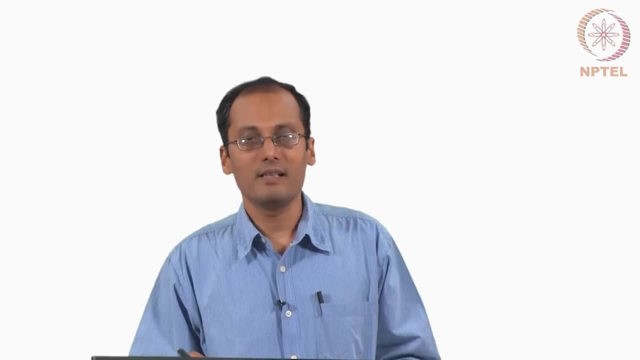 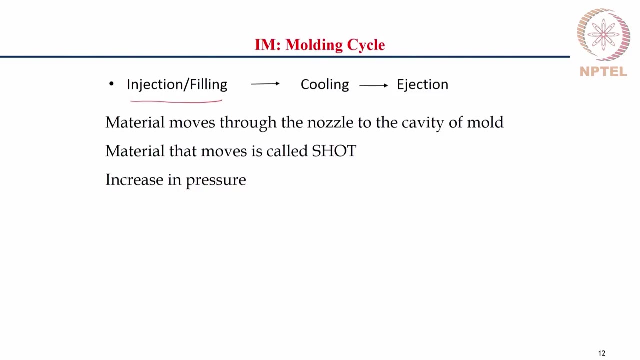 have a understanding of the mold cycle- injection molding cycle. So typically it consists of the filling stage, or what we call as the injection stage, and then the part cools inside the mold and then the part is ejected, So the material that is injected. 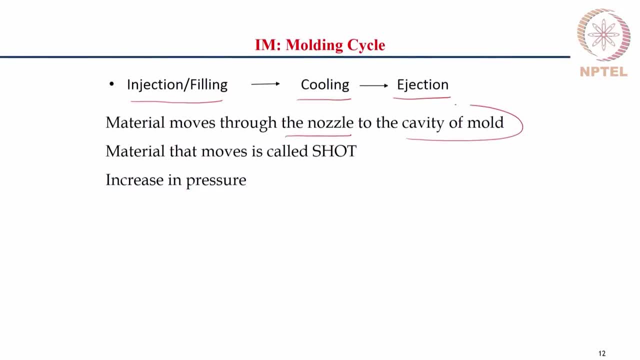 Injected through the nozzle into the cavity of the mold is called as a shot, and to make the material move into the mold we need to increase the pressure. So typically the injection pressure is the maximum while the material is injected and then gradually it is reduced. 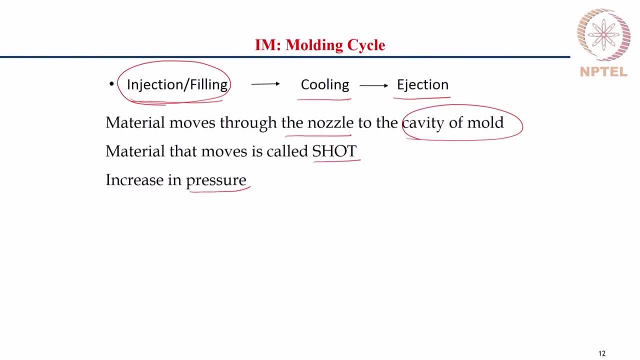 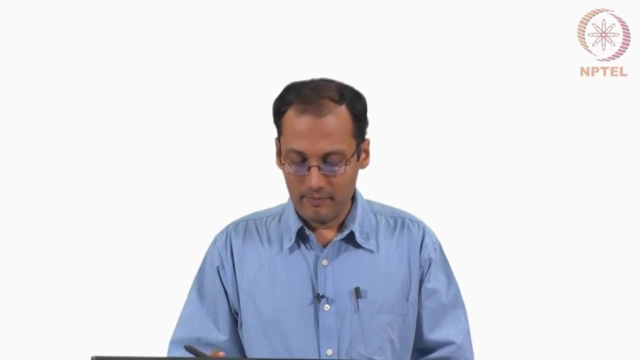 So this is the injection stage, While it is cooling and it is not there in part of cooling as well as in the ejection stage. So cooling is typically the longest period in one mold cycle because we need the material to cool and polymers being low conductive in nature, 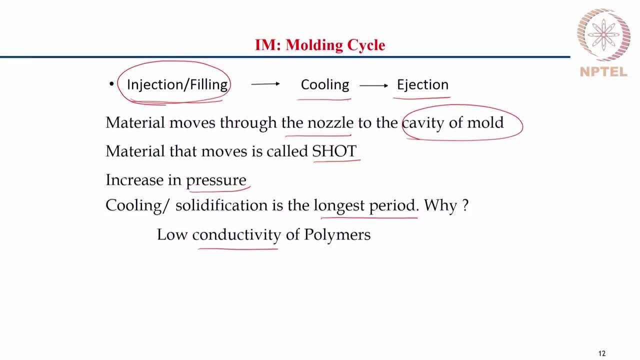 So we need to have the material to cool. So we need to have the material to cool. So we need to have the material to cool. So here we need to give more time for them to cool, Though heat sinks can be used to increase the rate of cooling. 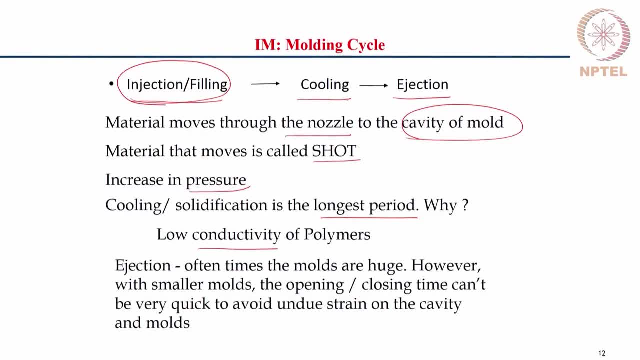 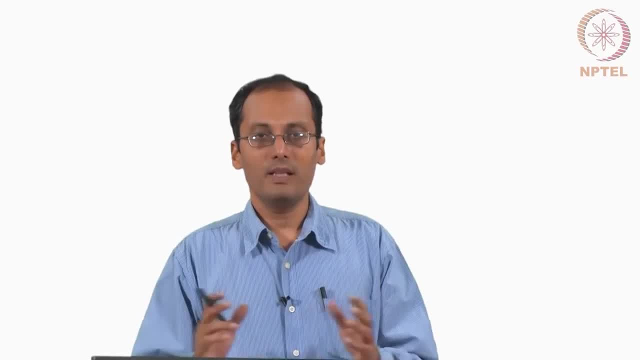 Ejection is the final stage, where the part is ejected from the mold by opening the mold, And there are also some ejection pins that are provided. So let us look at the final stage, where the part is ejected from the mold. Now let us look at the final stage. 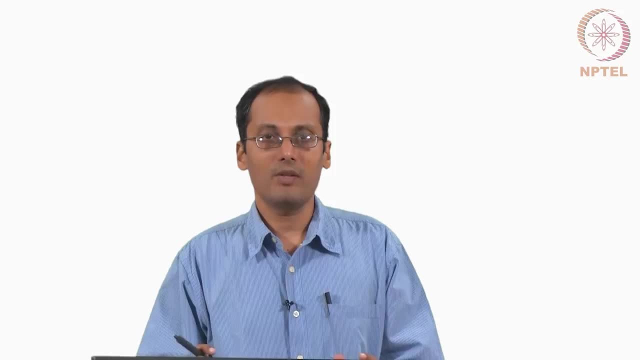 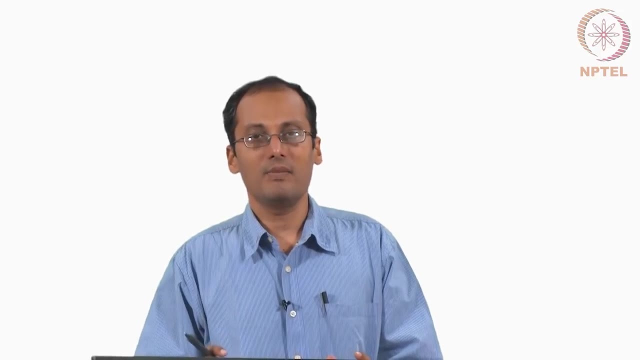 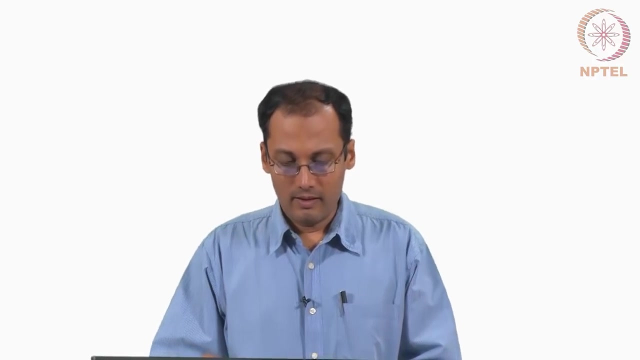 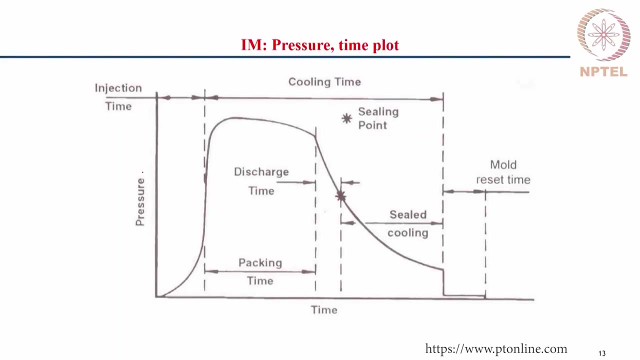 Ejection provided to help the part come out of the mold. drafts are also provided on the part surfaces so that the part can be ejected easily from the mold. So what we see here is the injection pressure versus the time associated with the molding. 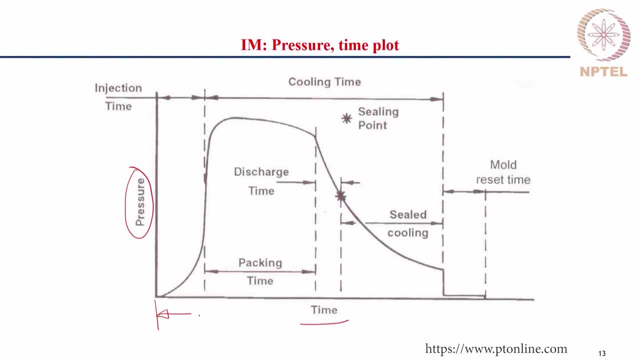 So what we see here is one full mold cycle which consist of the first part, which is the injection time, where the pressure gradually increases, and then the material fills the mold during this time, which is called as the packing time. And once the material fills the mold, the pressure is reduced. there is a point called as sealing. 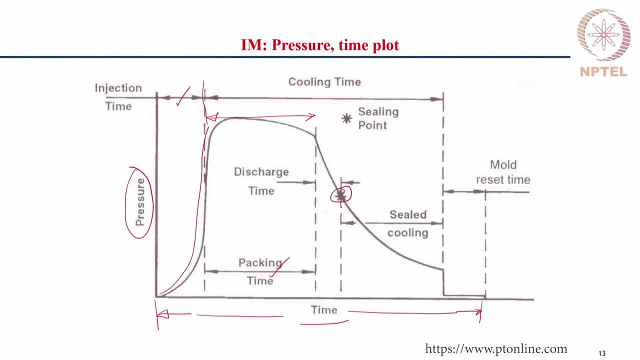 point where there is no further flow of material and the part is allowed to cool. in this sealed condition, Once the part is cooled, The part is ejected and it is reset for the next cycle. So this graph, which shows the injection pressure versus the time, is very important. from the 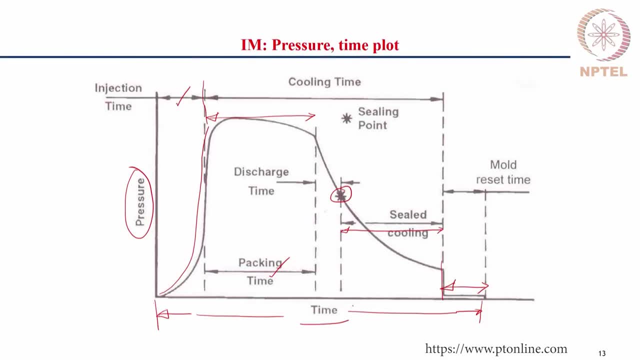 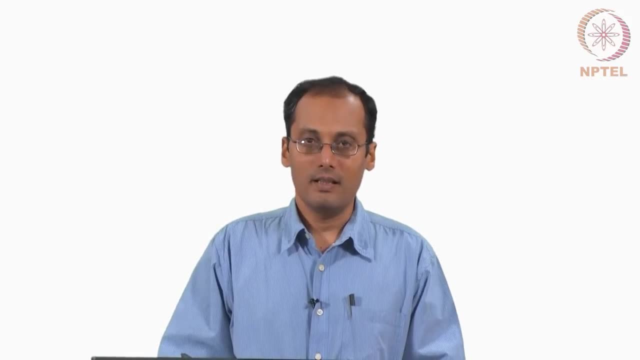 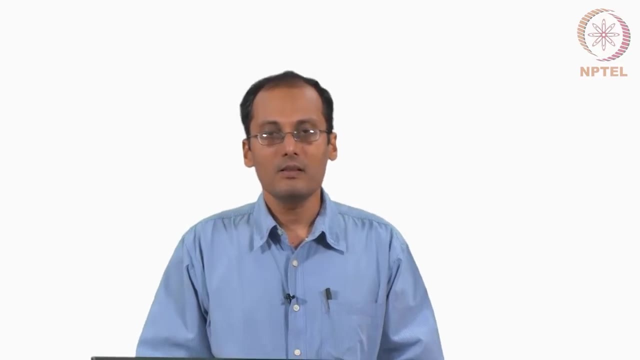 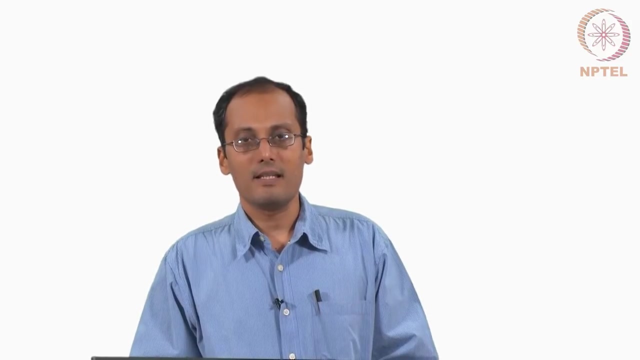 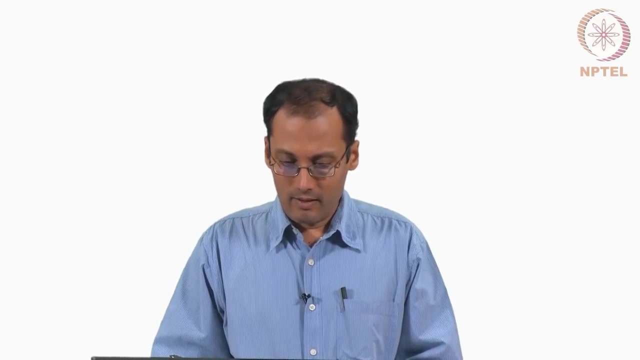 perspective of optimizing the mold cycle, And that is what we are going to discuss today, And thereby the cost of the component. This cycle decides the mold filling characteristics and thereby the part quality as well as the cost of the part. So this picture shows the injection molding unit. 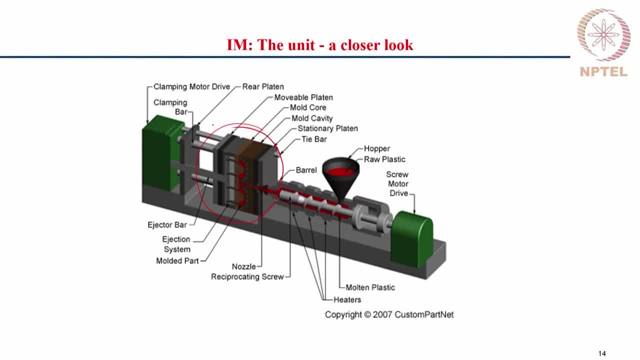 This is the mold and this is the injector. We have a nozzle here through which the material is injected. This is a hopper from which the material is fed, So there are heaters available in the injector which heat the material and the material flows. 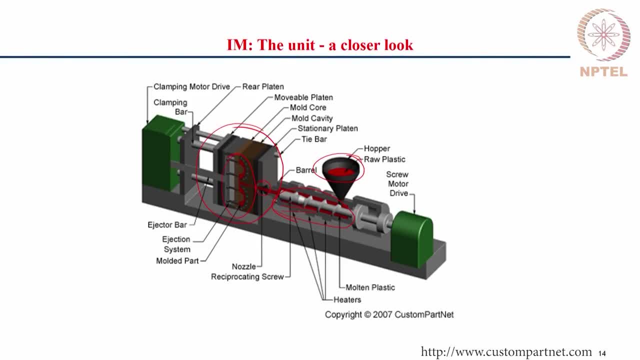 through this nozzle into the mold cavity. So the this side of the machine shows the clamping system, which applies the clamping force that is required to keep the two halves of the mold, This half and the other half, in the closed condition when the material is injected into. 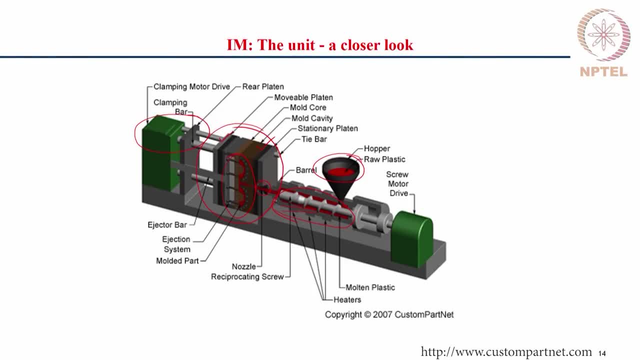 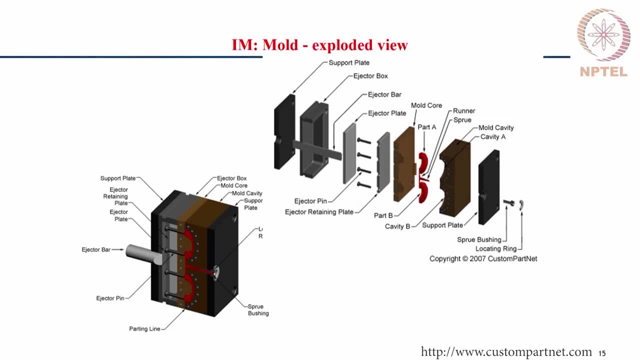 the mold. A closer view of the mold shows the details of the various components. So there are supporting plates which are clamped to the machine and which help in clamping the mold plates, The surface that divides the two molds, This is called the parting line or the parting surface, and on the injection side we have 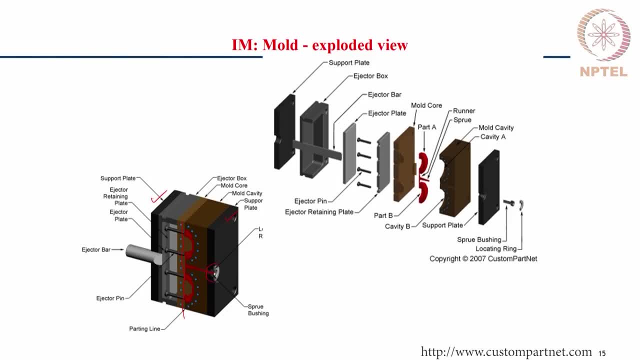 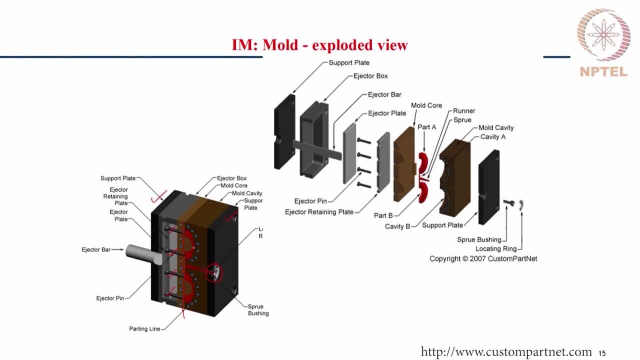 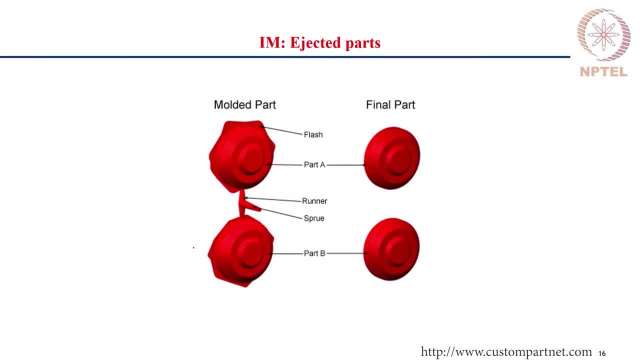 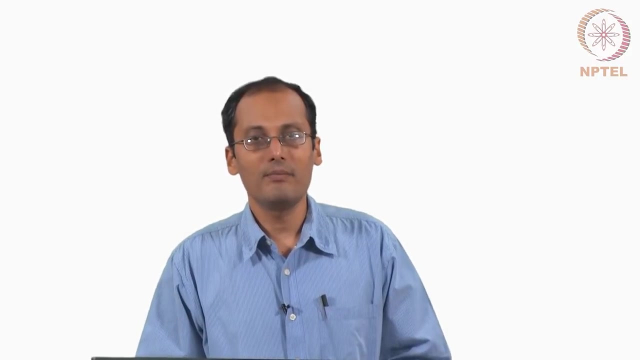 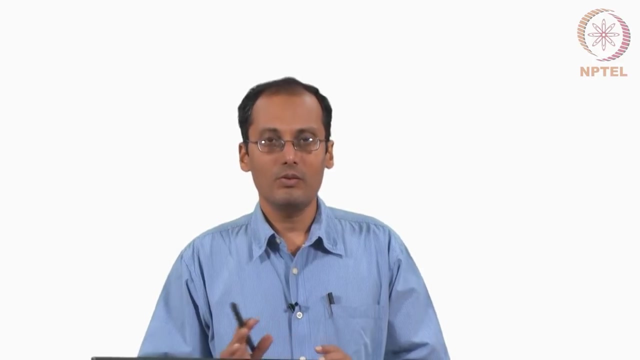 So this is the injection side. The part is completed When the part comes out of the mold or when the part is ejected. there are few unwanted elements associated with the part, like the flash. the flash is required because the flash the mold has completely filled and the material actually tries to come through the parting. 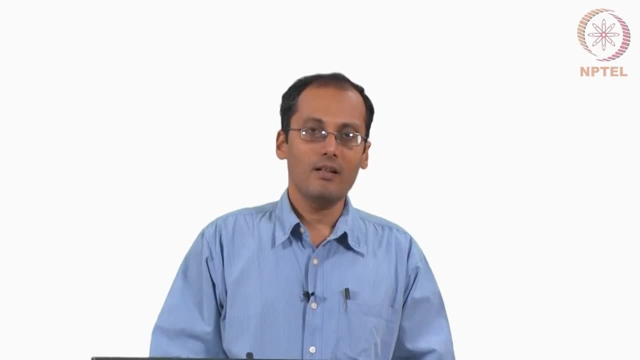 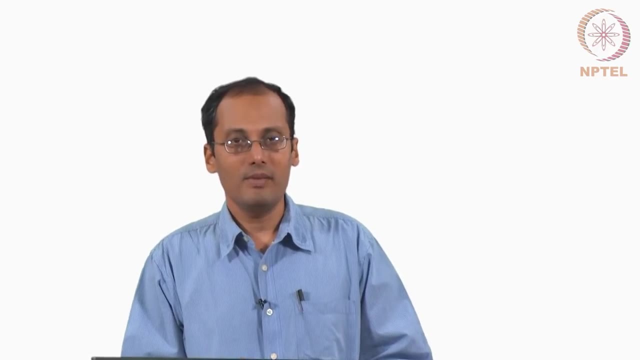 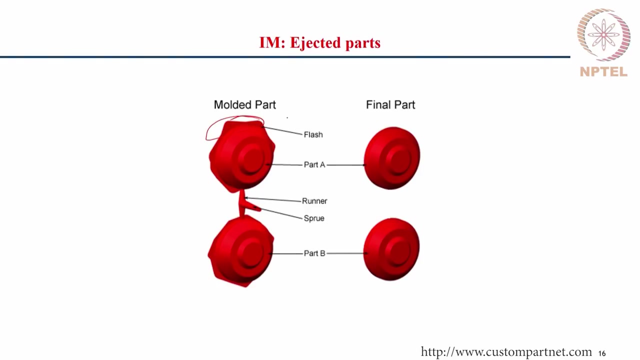 surface. This ensures that all parts of the mold are filled. So flash is an essential component, though it can be minimized but cannot be completely removed. Once the part is taken out, this flash is removed, as well as other elements like the runner, the sprues, and once these are removed, we have the final component. 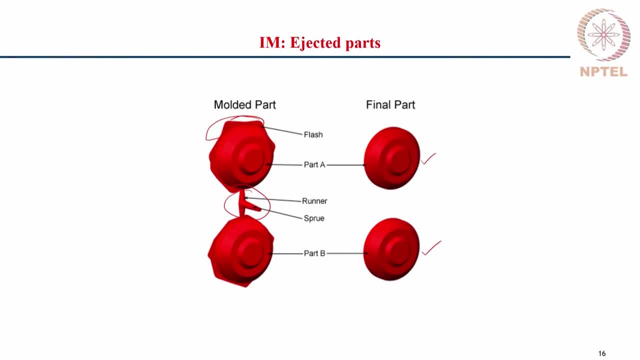 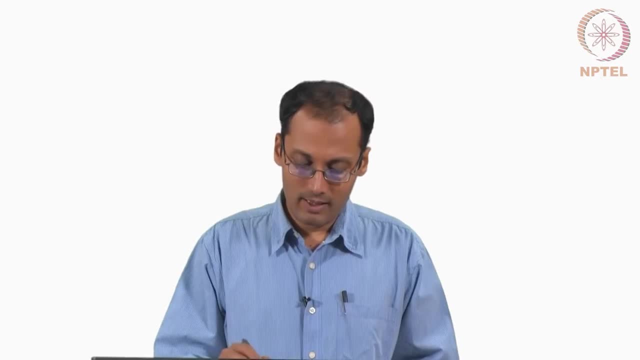 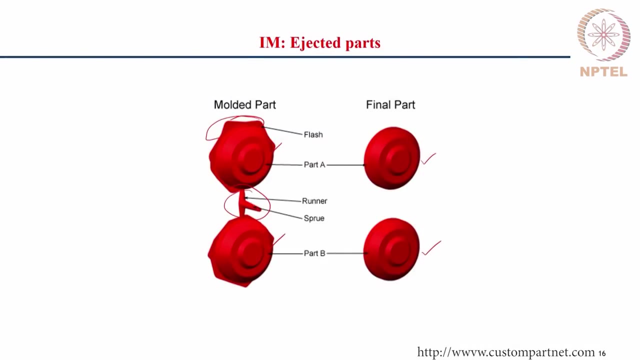 To reduce the part cost. typically, in a single mold there are multiple cavities, So each of this is a cavity, this is one cavity, this is an another cavity and to make the material flow to all the cavity, we have these runners on the mold which help in distributing the 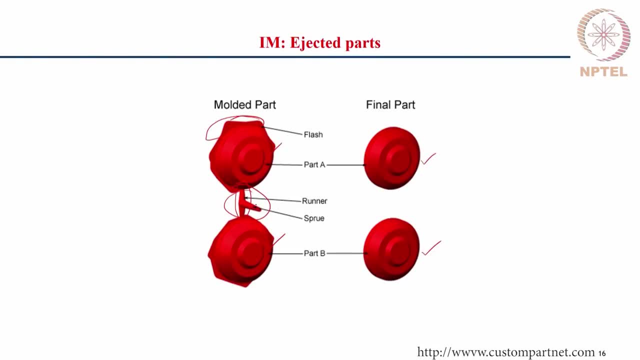 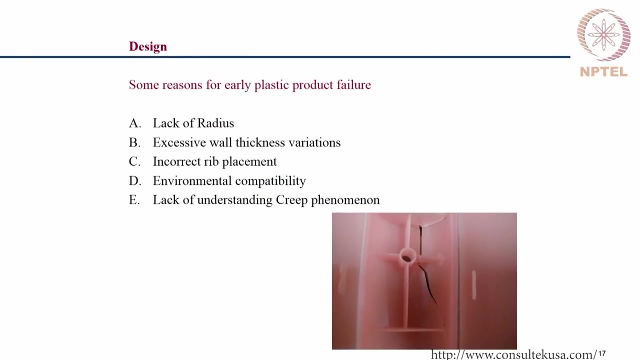 material from the injection sprue to the different cavities in the mold. Multiple cavities help in reducing the cost of the parts. While designing the mold, and as well as the selection of material and the design of the plastic component, we need to consider the typical failure that happens during service. 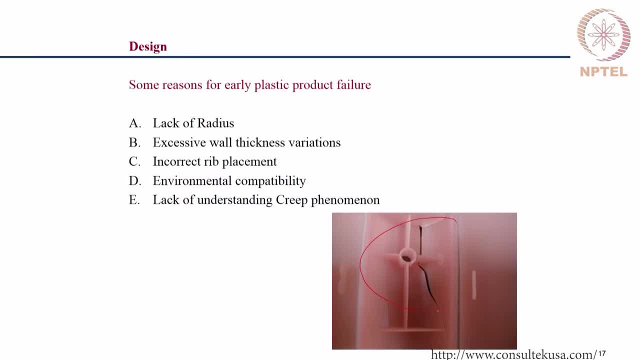 So in this slide you see a picture of a failure. This is a failed plastic component where the part has cracked because of the load that the part had to take, even though in the presence of stiffening elements like these webs or stiffeners that are available, 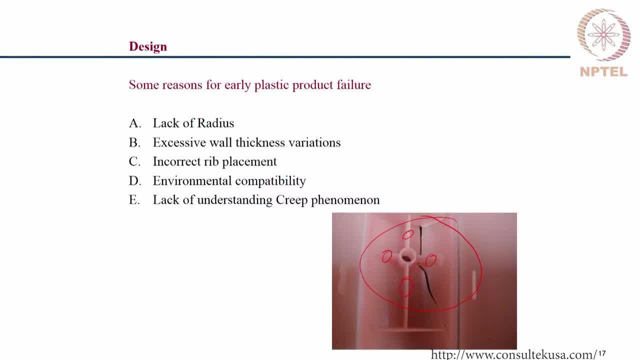 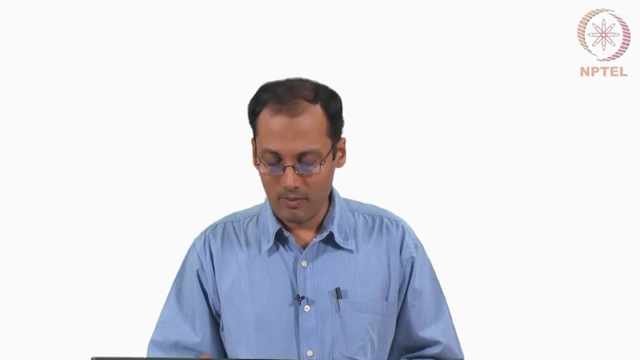 So some of the reasons for such failure could be that there is not sufficient rate of the material, the radius of the mold surface in the corners, which could cause the stresses to build up, or what we call as the building up of the stress, or stress concentration, because 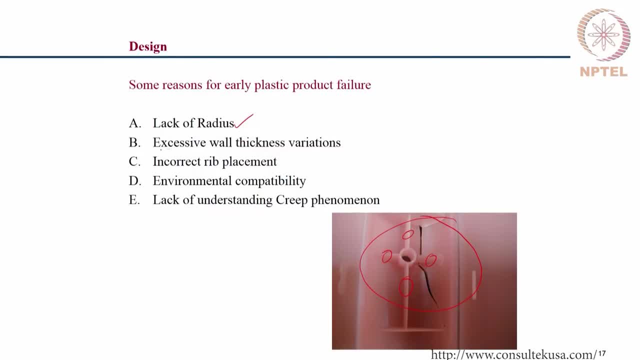 of lack of radius. It could also be because of excessive wall thickness. Where there is a slight edge to the material, there is no point in building the wall thickness. Because of the change in the wall thickness the material may not flow completely into. 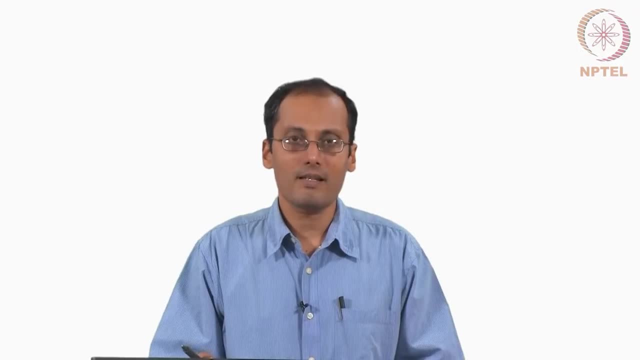 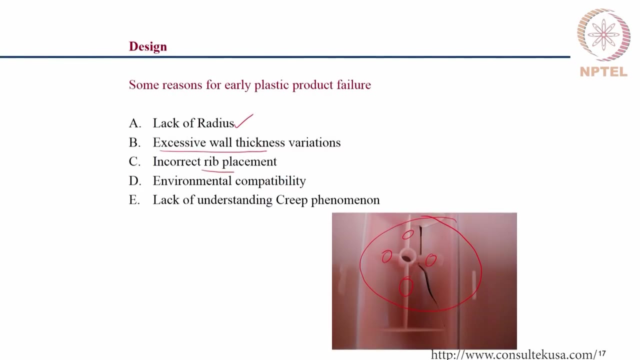 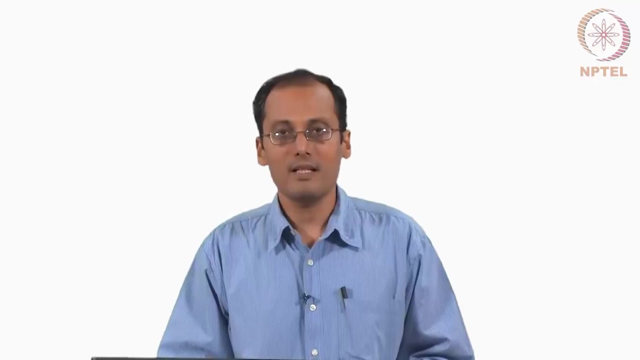 some parts or there could be differences in the stress which could lead to the failure. The placement of ribs are important. also the environment in which the component is serving. If the material is not chosen considering the various environmental conditions under which it has to serve, then also the component can fail. 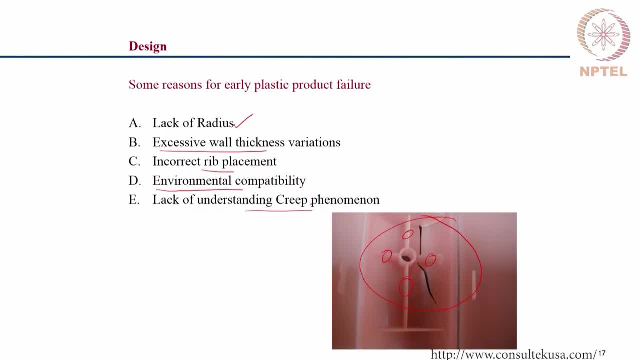 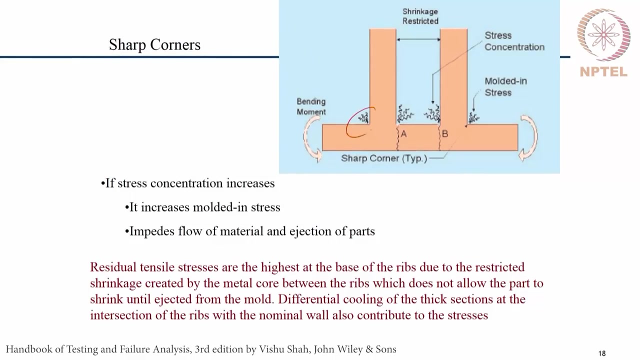 Also, material can fail because of creep, which is a long term failure phenomena. To avoid failures, one has to consider some design thumb rules While designing the plastic components we will see one by one. first thing is to avoid sharp corners or provide sufficient radius so that the stress concentrations can be minimized. 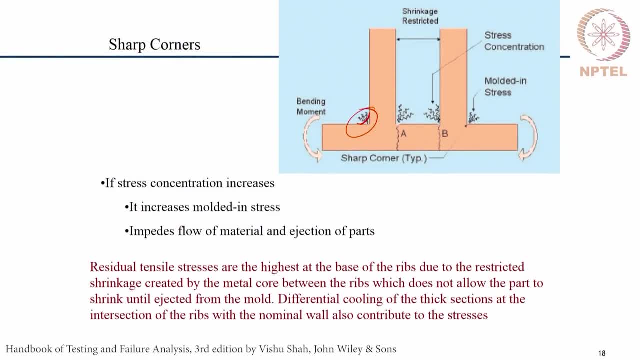 So wherever such stress, concentration happens, failure will happen. So the cracks can initiate at these points and the material or the part can fail. So at these points we have what we call as the molding stress, because the material has resistance in flowing at these corners. 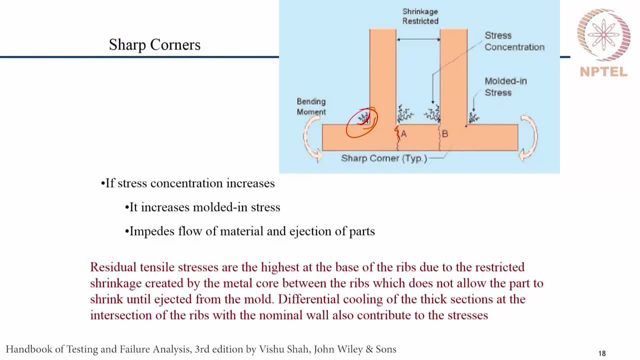 And that could happen, So the material can fail. So at these points we have what we call as the molding stress, because the material has resistance in flowing, So the material can fail. And that could also be a potential cause of increase in the failure because of the forces. 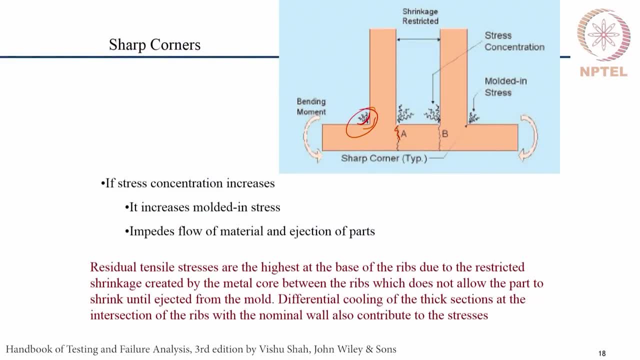 that are involved in ejecting this component Because of sharp corner radiuses the part, the ejection from the mold can also be a problem. So one of the important design consideration is to avoid such corners. So one of the important design consideration is to avoid such corners. 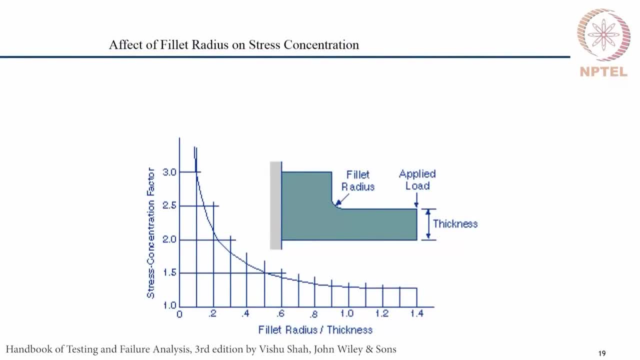 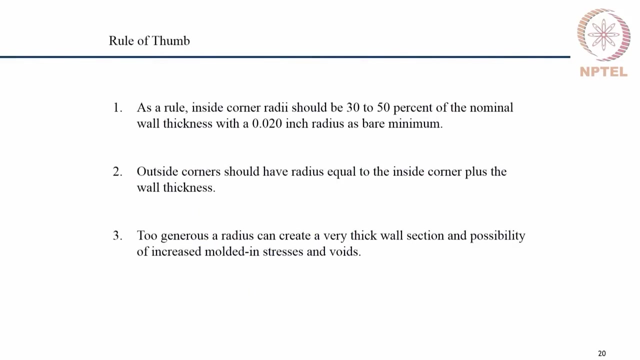 So one of the important design consideration is to avoid such corners. There are studies which reflect upon how this corner radius will have an effect on this stress concentration. So one can choose an appropriate radius and know what kind of a stress concentration factor one has to use in the design for any given applied load. 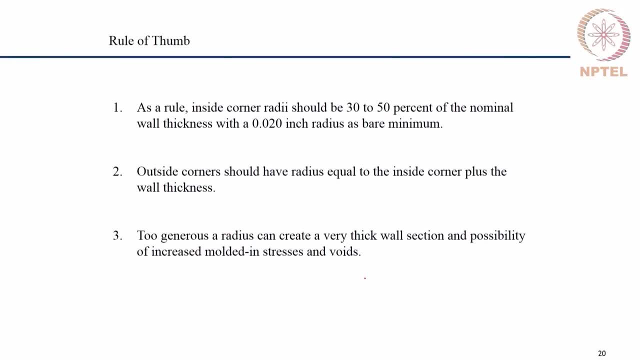 The general rule of thumb is to have an inner corner radius about 30 to 50 percent of the normal wall thickness. Say, if the normal wall thickness is 30 to 50 percent, then the inner corner radius is, wall thickness is t. the corner radius here r has to be about 50 percent of this value. 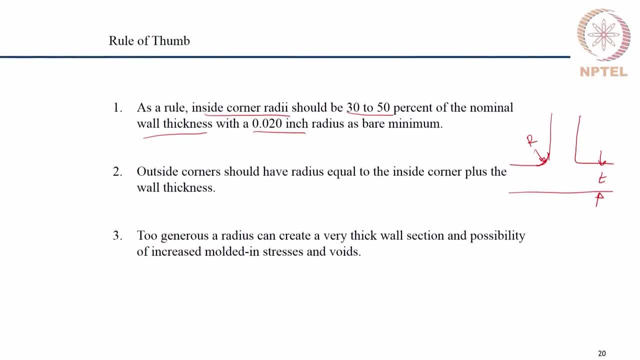 There are some suggested minimum value. Outside corners should have radius equal to the inside corner plus the wall thickness. So if there is a component like this, So this is the wall thickness, This is the inner radius and this is the outer radius. 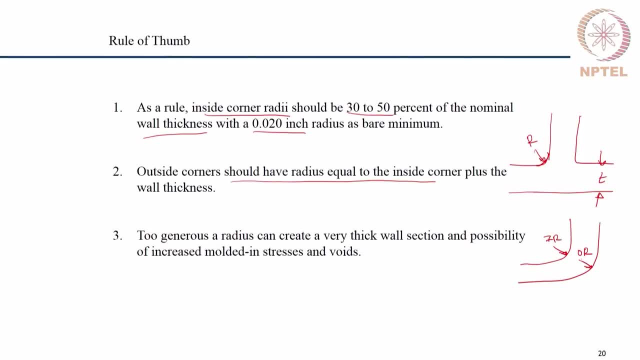 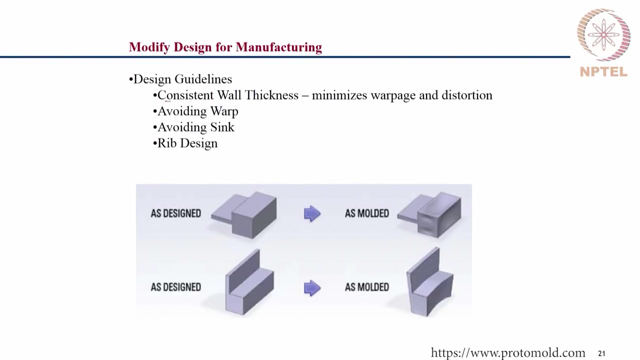 So once the inner radius is decided, the outer radius is taken based on the wall thickness and the inner radius. Too large a radius is also a problem because it will lead to lot of material and thereby shrinkage and warping. So when there are problems associated with changing wall thickness, the part shows warpage. 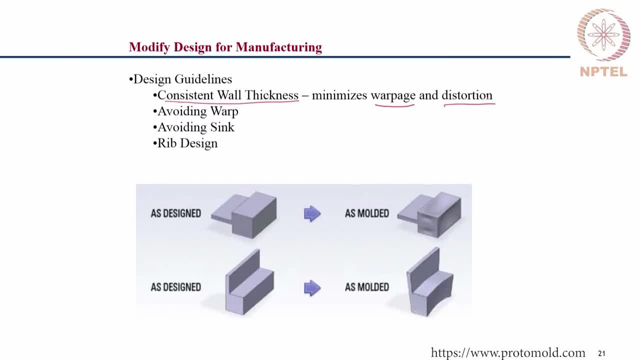 and distortion, as can be seen in this picture. So this is the designed component, or what is expected from the mold, But because of the change in thickness. so here the wall thickness is this much and there is a sudden change in the wall thickness, and because of which? because of this changed. 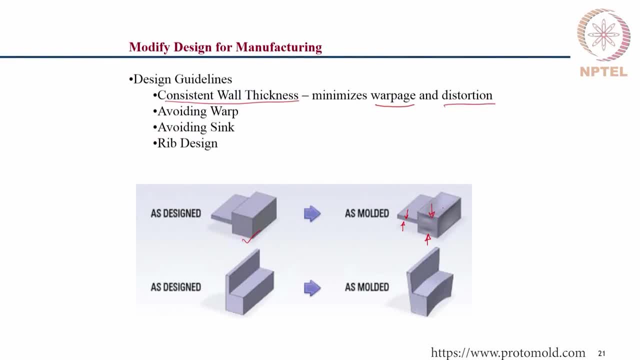 material. so there is warpage and distortion. So we can see the sink marks here and the warpage. So this is supposed to be a straight surface. instead it has warped. So by proper rib design and by either having constant wall thickness or gradually changing. 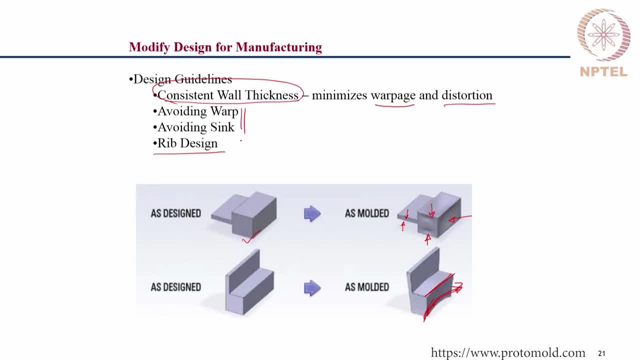 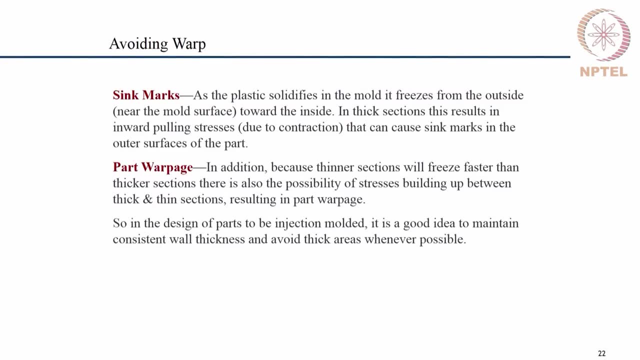 the wall thickness. these can be avoided, that is, warping and the sink marks. So we, as we saw, sink marks are caused because in the plastic solidifies on the surface, material is pulled inside and thereby the surface shows a sink mark. 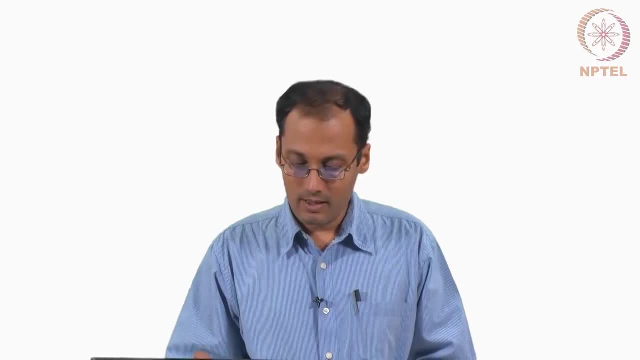 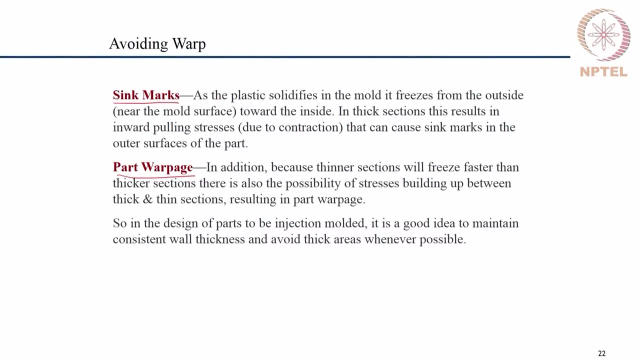 And the part warpage is again due to shrinkage. because a larger section is shrinking, it pulls a thinner section or it deforms a thinner section because of the shrinkage of a larger section. So these are typical problems associated with the plastic component. 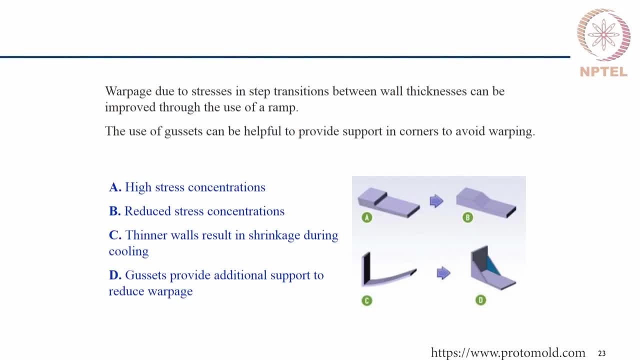 So warpage can be avoided by providing gussets. so these are the gussets Without gusset. the as designed component is supposed to be like this, but once the mold is done and the part is taken out, the part warps due to the stresses, and that can be. 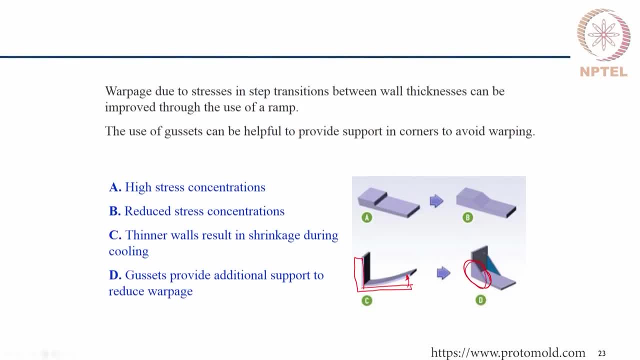 avoided by providing the gussets. And one can also avoid these steps, or what we call as change in the thickness, by providing a gradual change in the thickness. So these things can help avoid warping. So these are general guidelines one can follow while designing the mold. 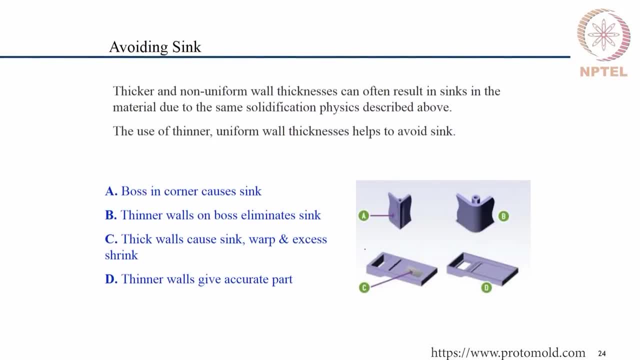 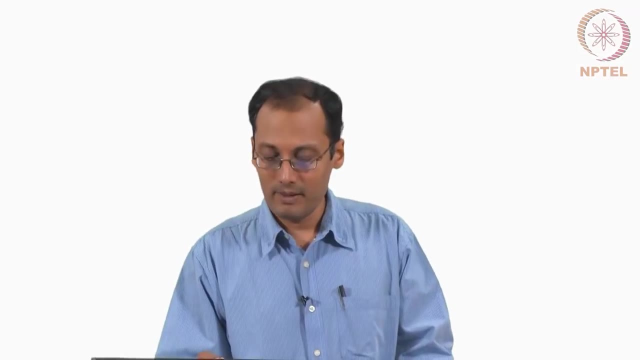 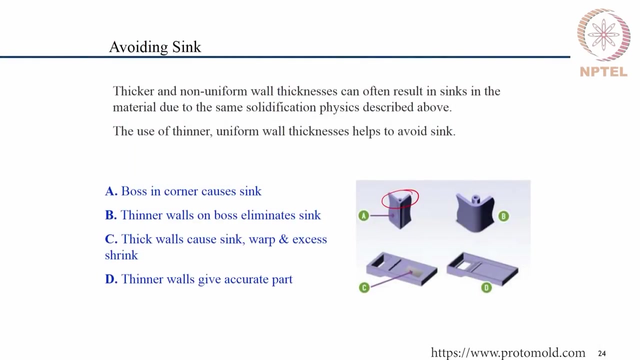 To avoid sink marks. one can use uniform wall thickness as far as possible. wherever it is not possible, one has to put design features that will help in maintaining uniform thickness. As we can see over here, there is a corner feature because of which there is a change. 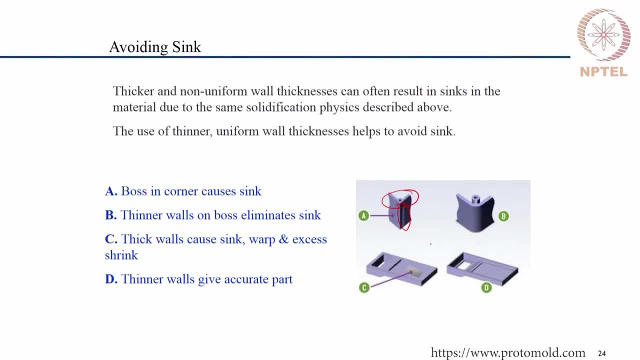 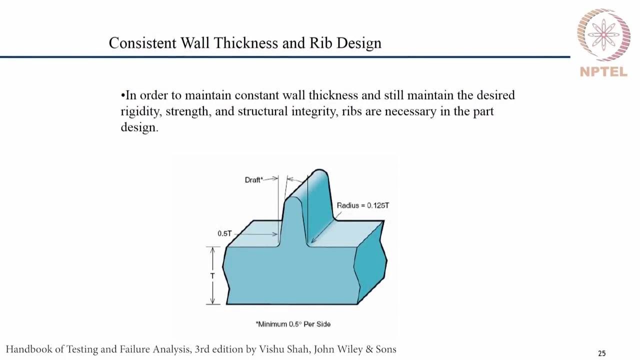 in the thickness and causing the sink mark. So we can change the design so that there is a constant wall thickness. I am just redrawing this for clarity So this thickness is kept uniform everywhere to avoid the sink marks. sections can be avoided wherever possible. 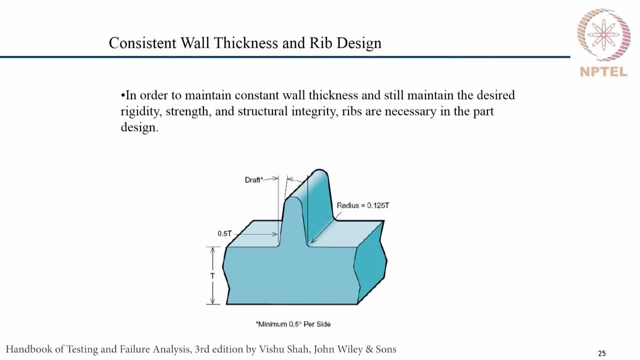 Ribs are to be designed properly so that one can avoid failures at these corners. So one of the important feature, dimension, is this corner radius. Based on this nominal wall thickness T, one has to make appropriate choice of this radius, the height of the rib and even the placement of the successive rib. 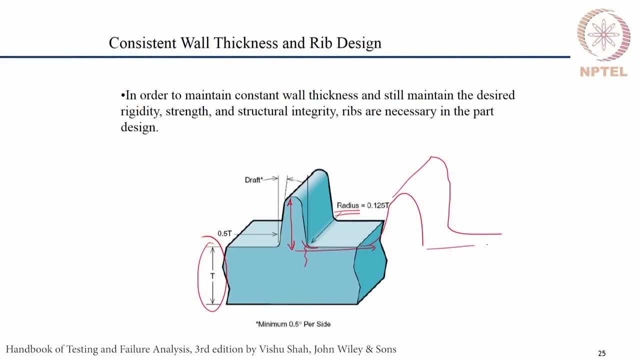 Let us say, if an another rib has to come here, What is the? The distance between the placement of two ribs, the height of the rib, the corner radius and placement of successive ribs. they need to be determined based on the nominal wall thickness. 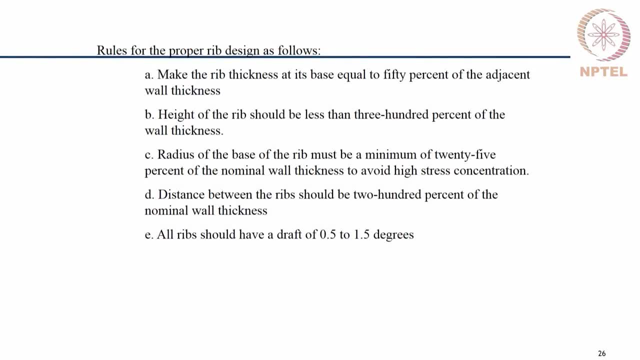 So there are guidelines to this. like the rib thickness is 50 percent of the adjacent wall thickness, The height of the rib should be less than 300 percent of the wall thickness, The radius of the base should be minimum 25 percentage and distance between the ribs should 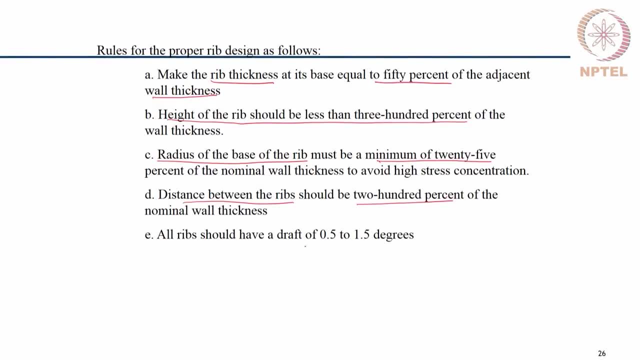 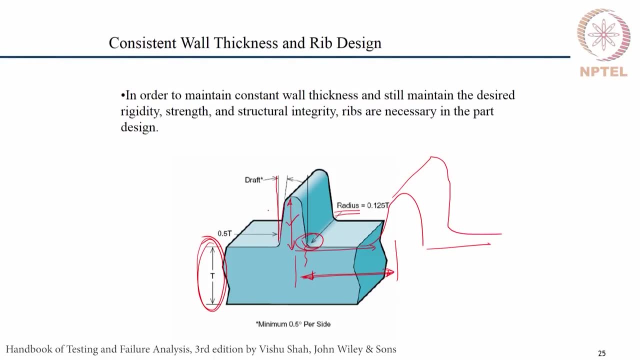 be 200 percentage and so forth, and there is also a draft. So this is the draft angle. This angle is the draft angle. This helps in removing the components. So the radius of the base should be minimum 25 percent and distance between the ribs should 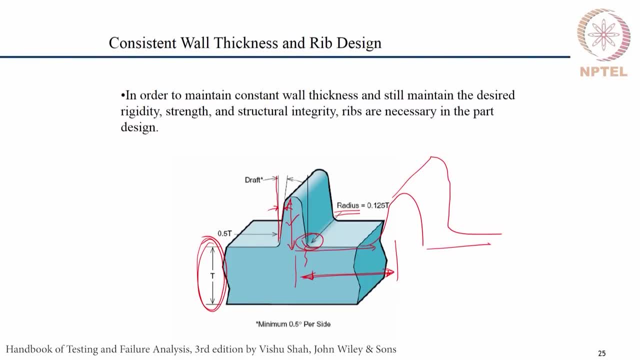 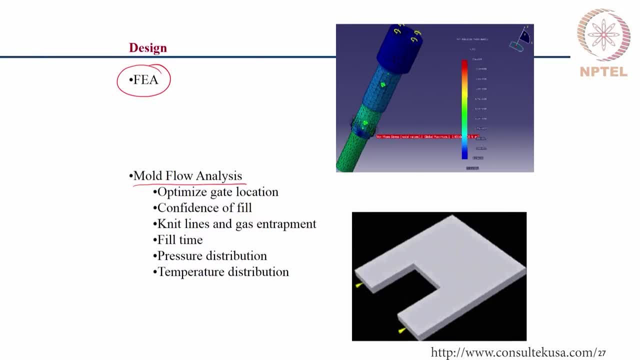 And it happens, analyzing how the mold flows into the, the material flows into the mold, the temperature distribution, the pressure distribution, all these can be studied numerically by computer simulation models, Finite element analysis, structural analysis can be done to understand the load versus deflection behavior of the design, the part, and one can change the design based on that. 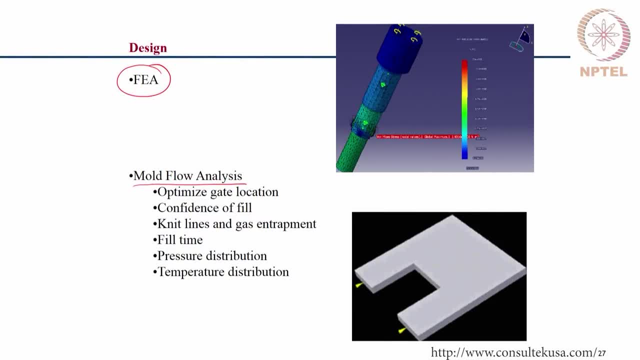 And for the designed component. one can do then a mold flow analysis to understand the process variables and its effect on the quality of the final component. So one can understand the fill time, because this is critical in terms of the mold cycle time and pressure and temperature distribution. 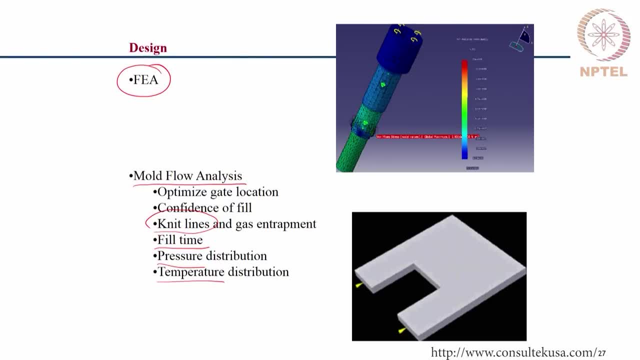 Also the formation of what is called as knit lines and gas entrapment, Like as an example in this picture. there are two gates through which the material flows into this cavity. So the material starts filling this cavity. and once the material fills, they will finally, 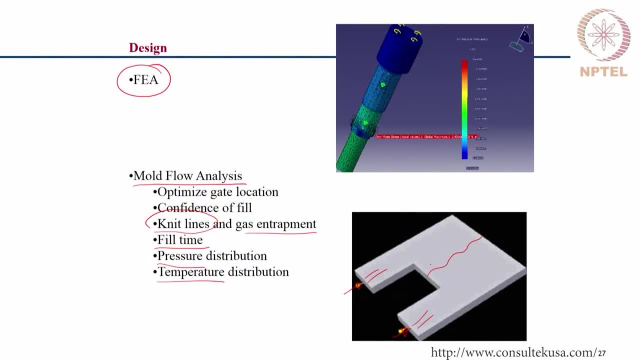 come and join, thereby forming These knit lines. so appropriate placement of these gates can help in deciding where these knit lines will happen. Knit lines should be avoided wherever there are high stress concentration regions. So by suitably placing the gates, one can decide or one can. 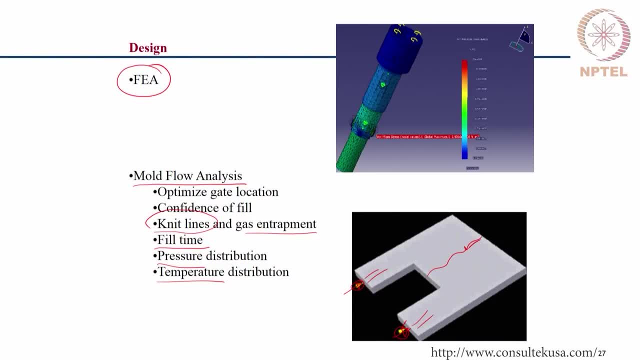 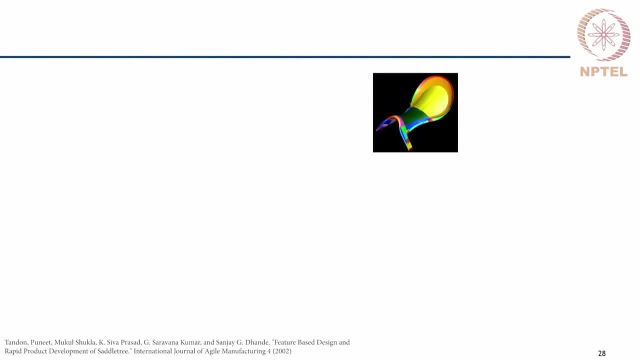 I get the knit lines at places where there are no high concentration of stresses. So this is an example design process which I am showing using one product- This is called as a saddle tree, which is used in the saddle which is main, you know, a leather. 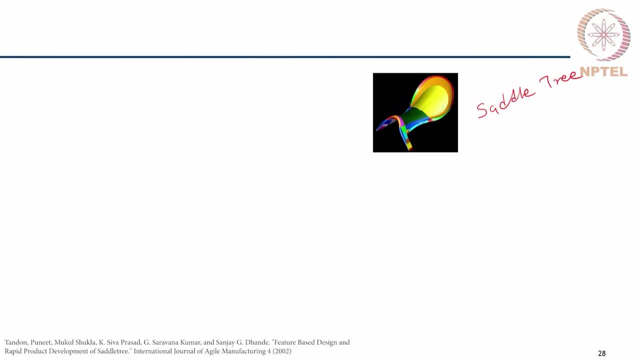 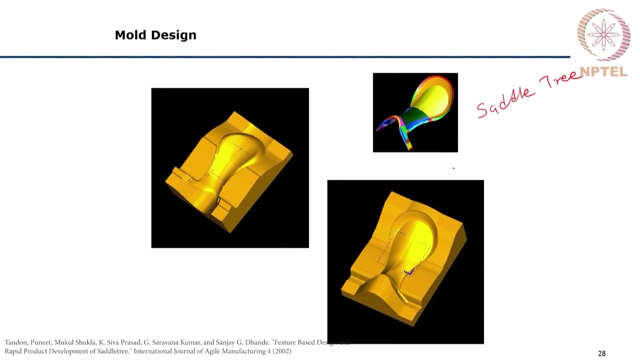 component used to help jockey sit in a on a horse while riding. So this is a saddle tree, which is a injection molded component. What you see is a CAD drawing and, based on the CAD, one designs the mold. The two halves of the mold are shown. 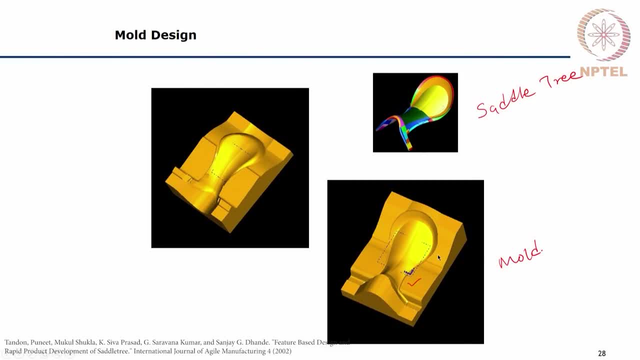 This is the parting surface that you see And this is the cavity. So there are softwares available to help do this mold design. once we have the part design From part design, we get this mold design. Ok, Ok, Thank you. 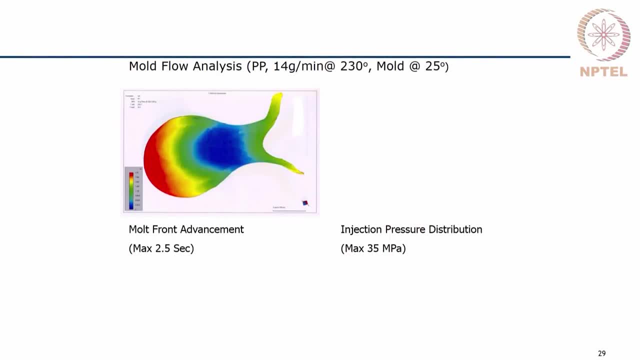 Once we have the mould design, we can use suitable softwares to do the mould flow analysis, Like here. you see a simulation of polypropylene being injected at 14 grams per minute rate at this temperature, mould being kept at 25 degrees. 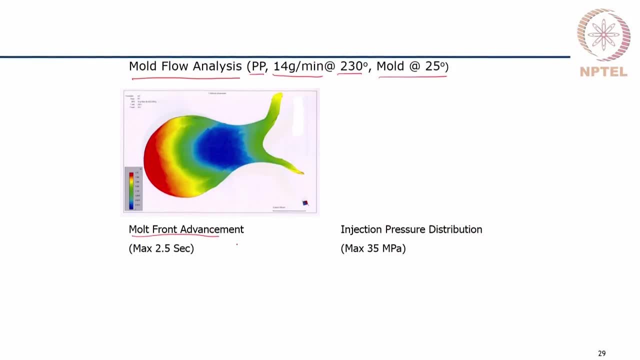 It shows the mould front advancement, how the material flows from the injection point which is over here, to the different regions. So one can see at different times how the material flows into the cavity. what are the regions which get filled up at the last, like here? we say that it takes almost 2.5 seconds. 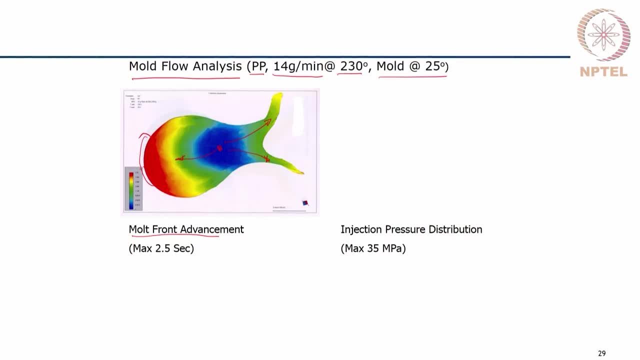 to fill For the material to reach here, whereas it is only about 1 second somewhere over here. One can also analyze the injection pressure that is required for filling this cavity and its distribution. Injection pressure decides also the capacity of the mould holding force that is required. 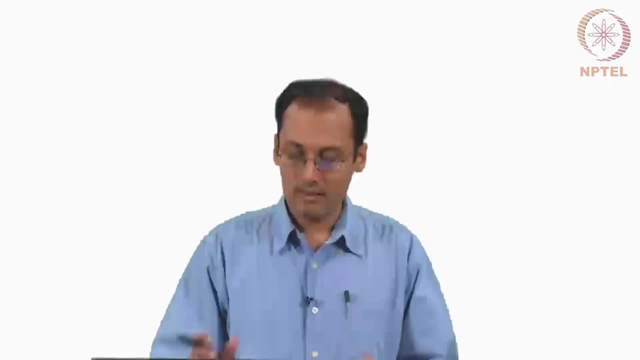 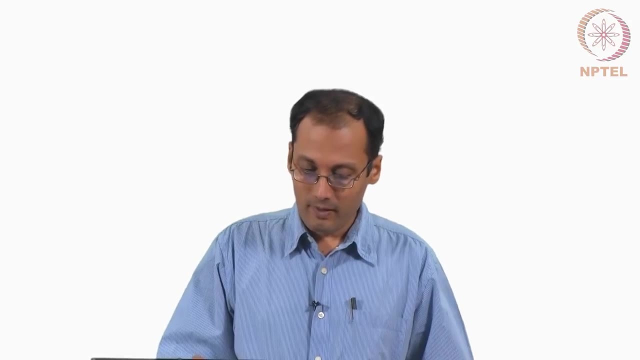 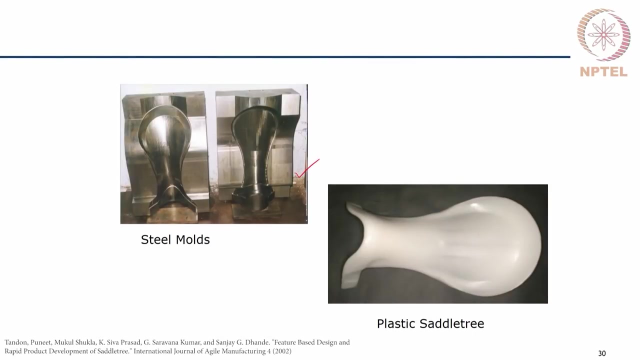 and thereby the capacity of the machine itself to hold the or to provide the clamping force that is required to hold the moulds together. These are pictures showing the finally manufactured tools. Once these simulations are done and the design of the mould is verified, one can go for production. 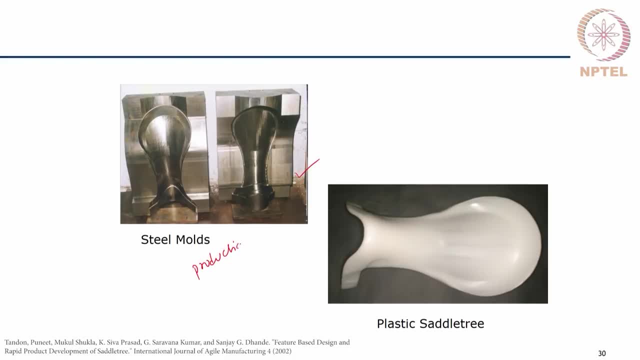 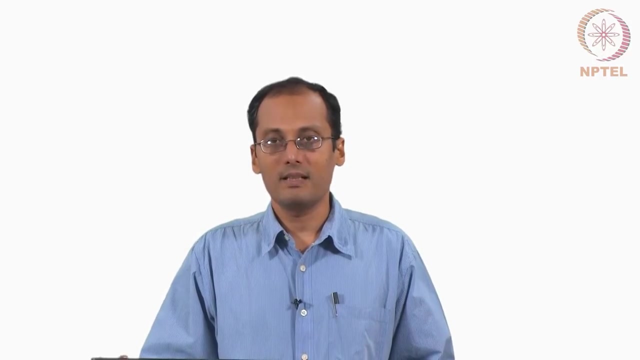 tools And we have the production parts coming from that. So we see that the design of the mould is critical from the perspective that the material has to flow. We need to optimize the filling time- Ok, or what is called as the mold cycle time- so that the cost is kept at the minimum.